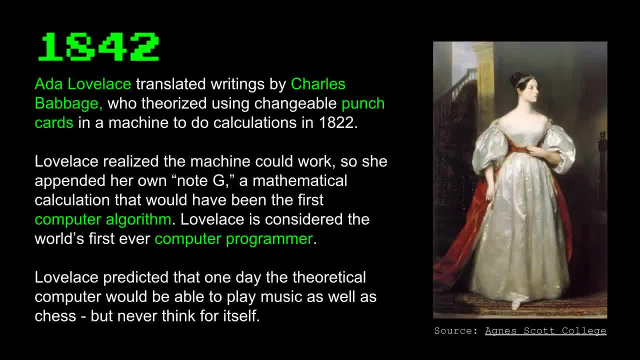 Back in the 1800s punch cards. Remember that It's going to come up again Now- a woman named Ada Lovelace. it all goes back to Charles Babbage, like in 1822.. He came up with 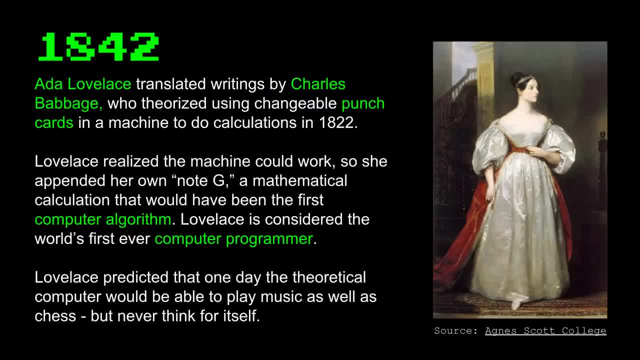 the idea of using these punch cards that were already used in the textile industry. He goes: why can't I make a calculator with these punch cards? And the thing is he could. A little bit later, on 1842, Ada Lovelace was charged with translating Charles Babbage's writings. They 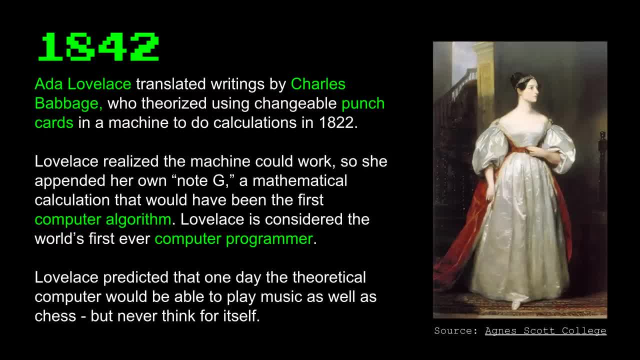 actually knew each other. They used to meet and talk about this punch card thing and the theories. So she realized: hey, you know what This machine could work, even though Charles Babbage couldn't really build it at the time, because the technology 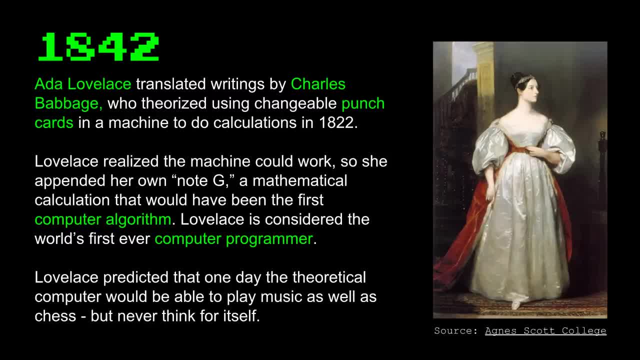 either didn't exist or was too expensive, one reason or another, and they never built this thing back in the 1800s. But she appended her own little note to the translation for this mathematical calculation that would have been the first computer algorithm, So the 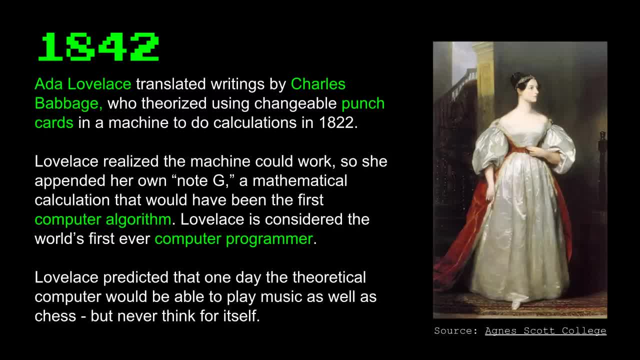 industry kind of widely considers her the first ever computer programmer. That's right, ladies. A woman was the first ever computer programmer. That blows the glass ceiling off the building, doesn't it? Lovelace predicted that one day the theoretical computer would be able to. 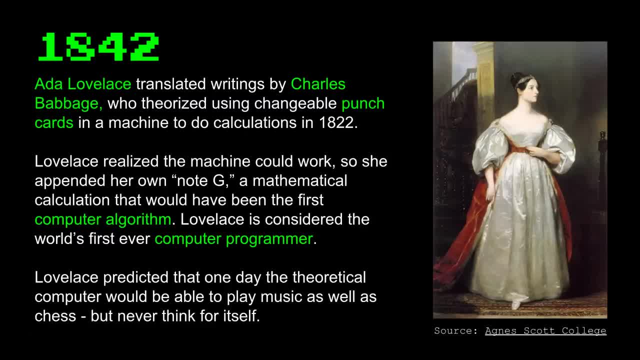 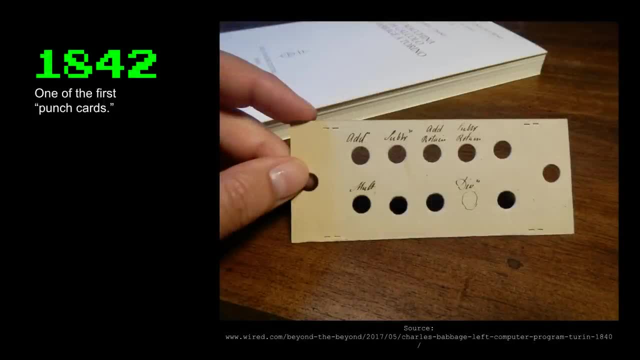 play music as well as chess. Yeah right, Never happened, right. But she also said that a computer would never think for itself, And we are beginning to take the wraps off of that right now here in the 21st century. So we'll see how that pans out. Here's one of the first punch cards. 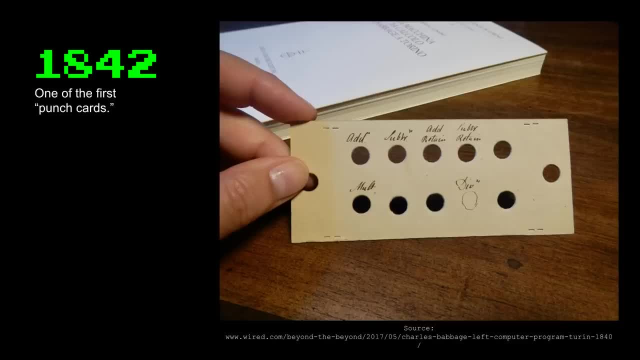 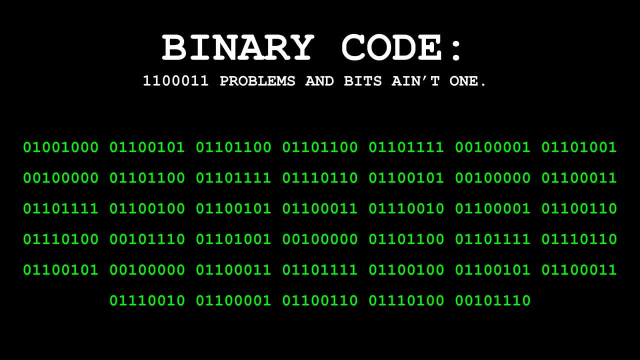 supposedly created by Babbage. Now Babbage uses the base 10 system for his machine, from what I understand, And it wasn't really the best way to go, as we'll find out a little bit later. So what are we using? computers? We've got 1100011 problems That. 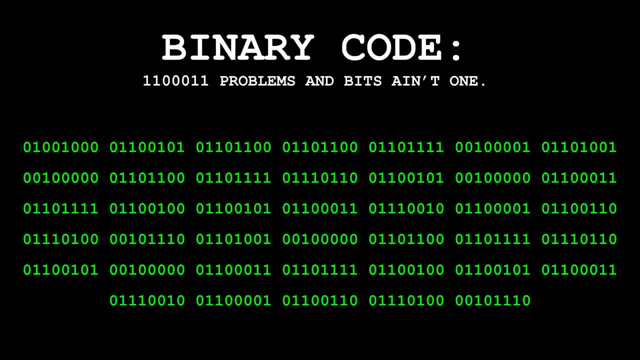 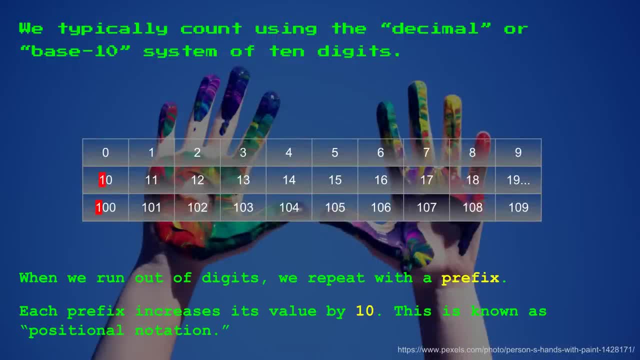 translates to 99 for those binary geeks. And bits ain't one. You get it. 99 problems and bits ain't one. So what is binary code? We typically count using the decimal system or the base 10 system of 10 digits. Why? Probably because we have 10 fingers. Who knows? We can't go back that far and 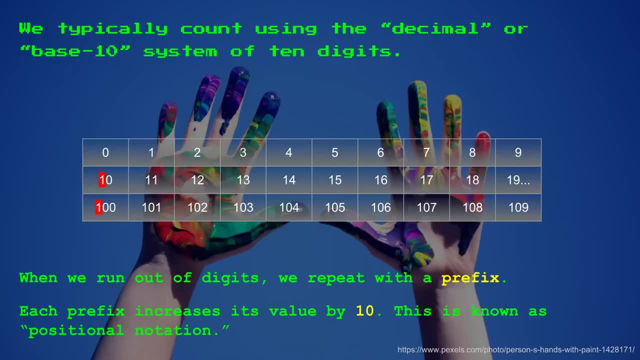 ask the guys back in wherever it was that came up with this thing. You know, probably in the Middle East somewhere, saying, hey, why do we use the base 10 system? Well, we don't know, But check it out. We go from zero to nine, So we have 10 digits. We start with zero. 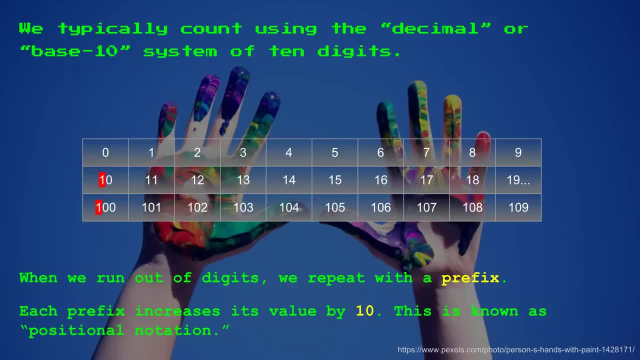 not one. We go to nine. And then what happens? when we hit nine We run out of numbers, right, So we got to roll over. So we use something called a prefix or positional notation. We add a one, So we go from zero, then we go from nine and 10 and 100 when we run out of those digits And 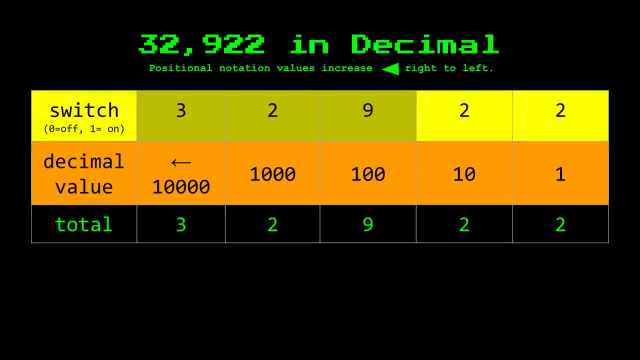 you know, that's how we count. It's called base 10 or the decimal system. So what is 32,000?? It's my zip code: 32,922 in decimal We go from right to left. You see the. 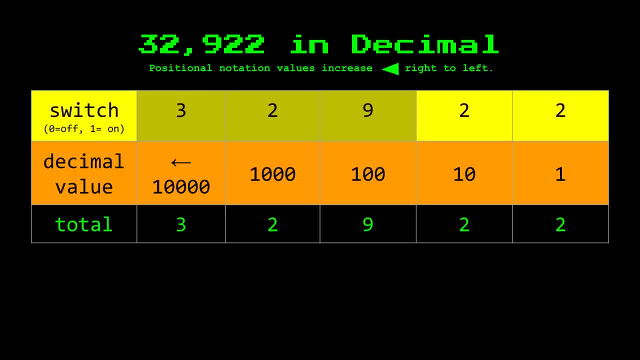 positional notation values increase by a value or a power of 10 as we go further to the left. So we start with the ones and the tens: 100, blah, blah, blah. So we know that 32,922, we add up all the. 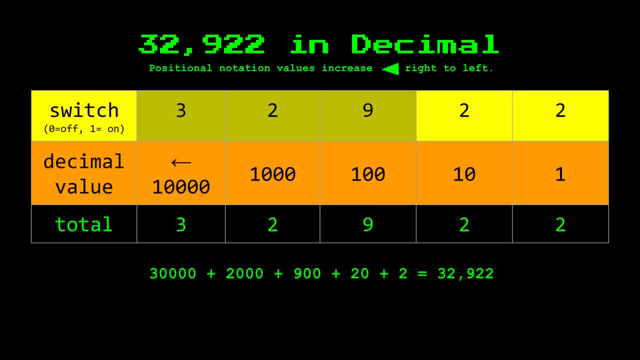 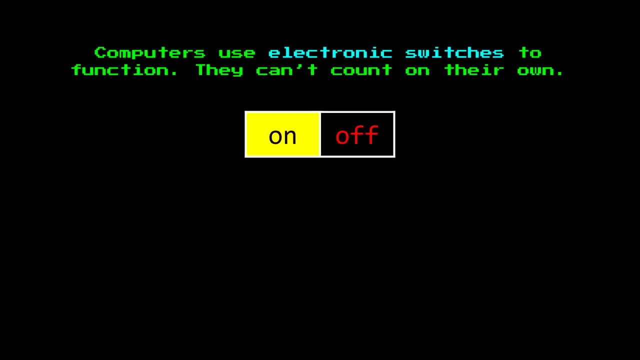 positional notation, all the values in those little buckets, comes out to 32,922.. Get it, Makes sense. Base 10.. Well, computers use electronic switches To function. They can't count to 10. They can't count on their own Computers. 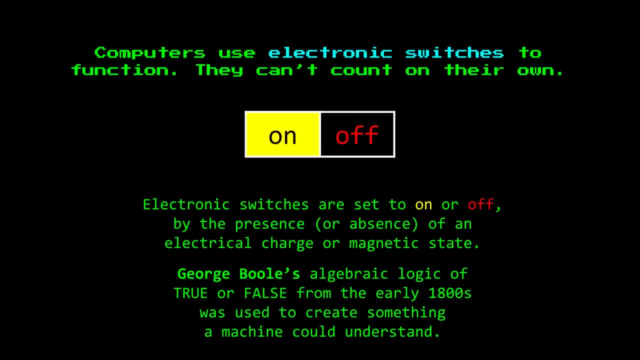 are inherently stupid until people tell them what to do. I know it's hard to imagine a computer being stupid, especially when you have these fantastic things like Siri and Alexa being able to. we'll go into that later how that's even possible. It's nuts, But electronic switches. 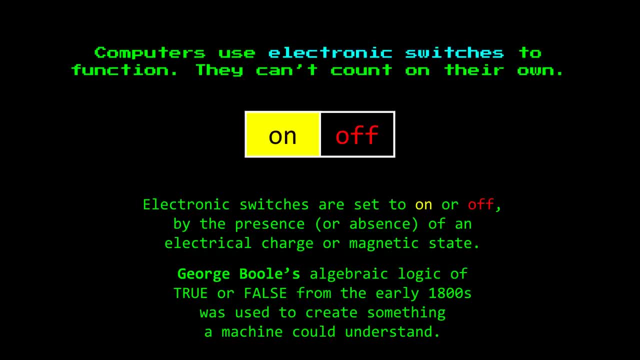 think: on and off We've got a voltage or we have no voltage. That's actually oversimplifying, because we either have a higher voltage and a lower voltage. We either have a higher voltage and a lower voltage or a mid-range voltage that's kind of thrown away, or no voltage at all in some. 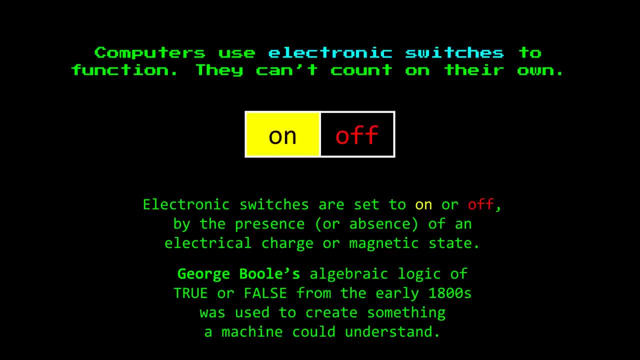 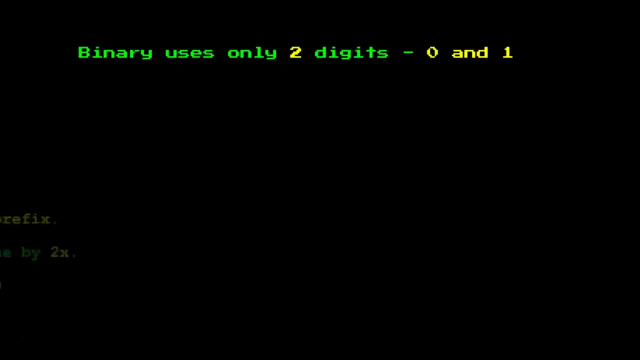 cases, But I don't know. It goes back to George Boole's algebraic logic, again from the 1800s, of true or false. Supposedly he could use his algebraic logic to figure out any problem, any mathematical equation, using just true or false statements, And it wasn't the most efficient. 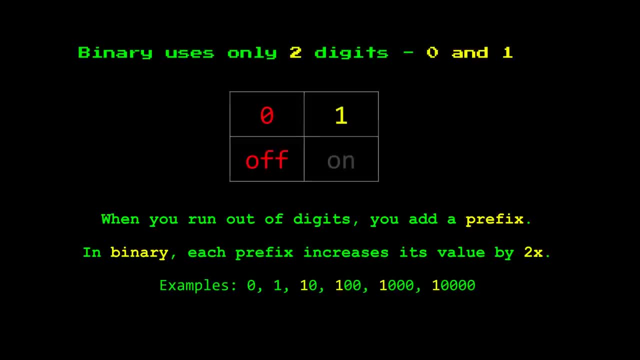 thing, but hey, it worked. So binary is different than base 10.. It only uses two digits. The only two digits you will ever use is the base 10.. And that's what we're going to do. We're going to. 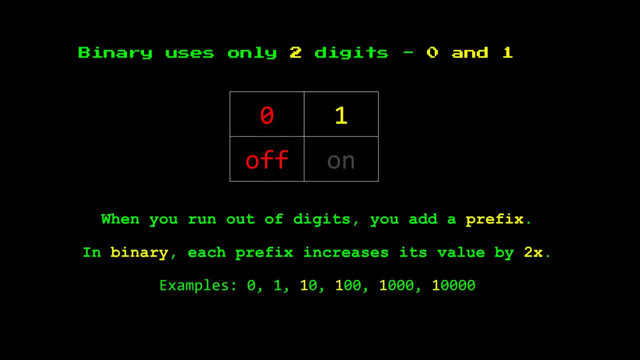 see in binary is zero or are zero and one, And zero indicates an off state and one indicates an on state. And then, when you run out of digits, you add a prefix. But what's your prefix? Well, in binary, each prefix, you add that one to the beginning of it. it increases its value by two. 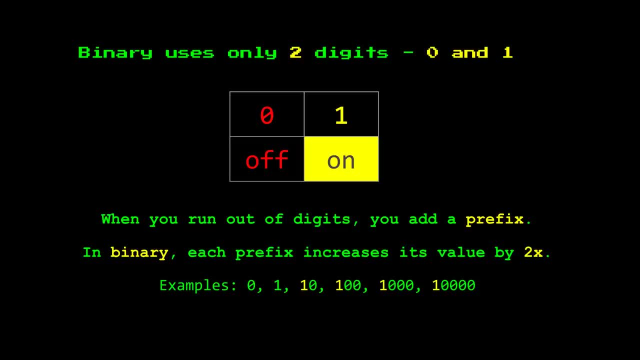 times You get it Because you only got two digits. You can't increase it by 10 because you don't have 10 digits, You only have two. So check it out. This is how it works. This is zero to four. 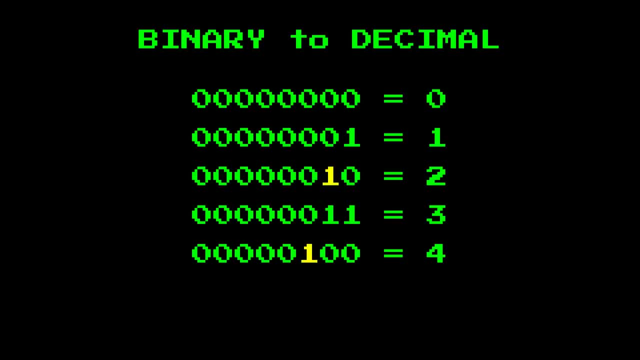 in binary On the right you see decimal On the left you see the binaries. You see if you go, zero and one are the same, But then you go to the number two. No, you got to use that positional notation You. 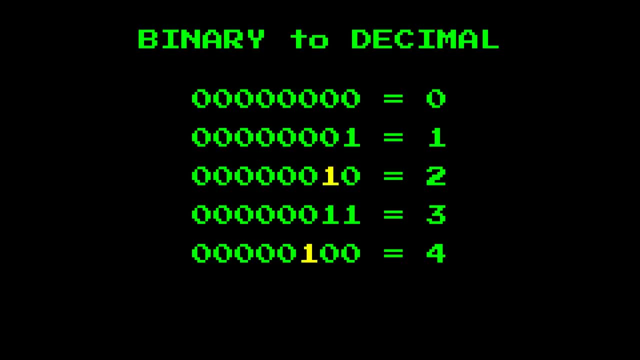 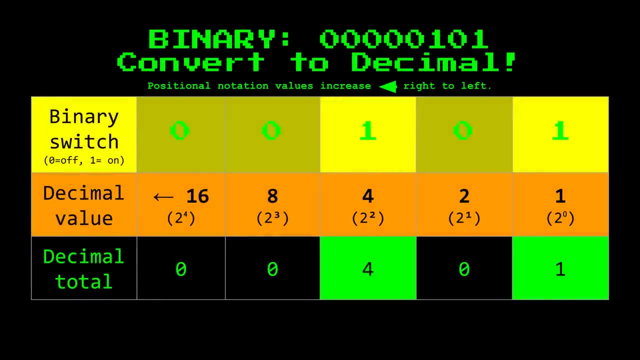 got to put a one there because you're running out of numbers, right, And then three is one one, And then four we're going to bounce out again, So you can see how these numbers can get tediously crazy long. So let's do a simple conversion. We're going to take zero, zero. 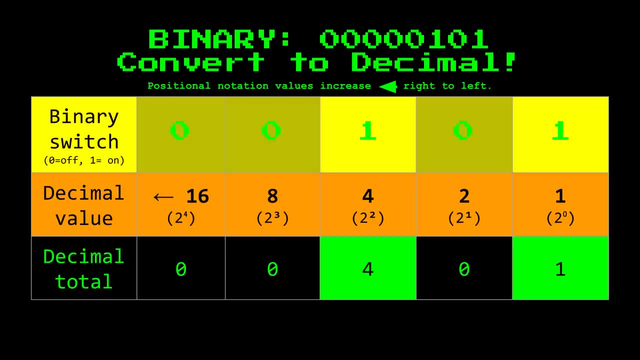 zero, zero, zero, one, zero one. converted to decimal right. Remember positional notation: values increase from right to left, So we're going to the left here. Decimal value: in a binary situation it's going to increase by one power of two. So any number. 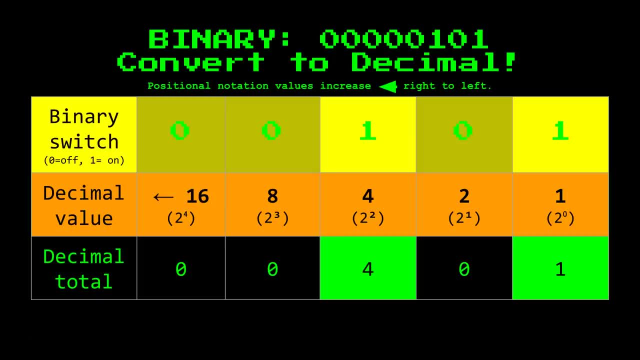 to the power of zero is one. You remember that from grade school math. I didn't, I had to look it up. And then we go to two, to the power of one. right, It's going to be two. and then two to the. 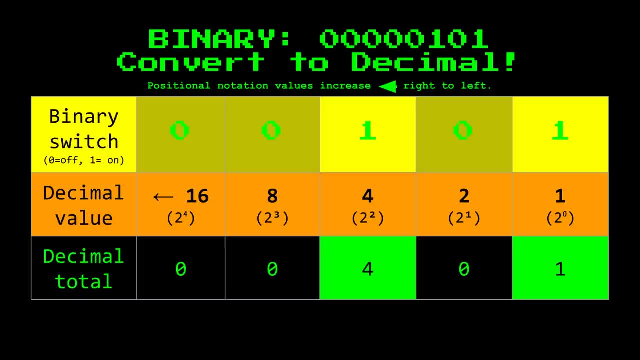 power of two, four, et cetera, all the way down the line. So what's one, zero, one? When we look at the switches here, think of these numbers, these binary numbers, as switches. They're on or off, remember, And a one indicates the switch is on. 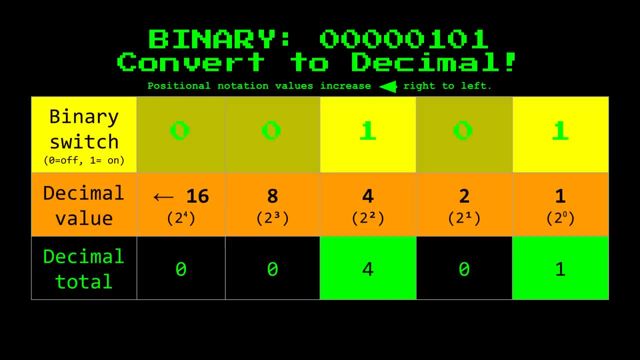 A zero indicates the switch is off. So we have two switches in the on position right, Then the ones column all the way to the right. the one switch, two to the zero power. the value of one in decimal is on. We go one to the left and that second position's off. So we don't count it. We. 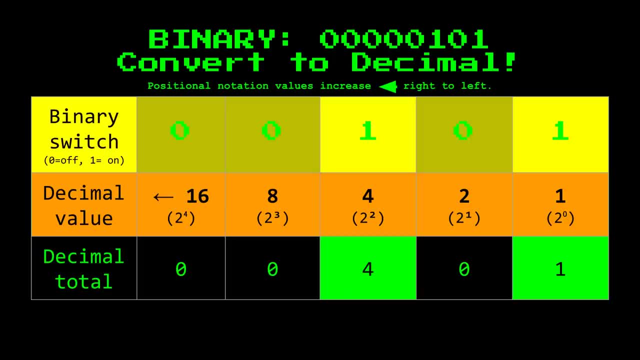 go one more over. Oh, look, look, look look. Position number three is on. It's two to the second power, two to the two power, which is four, So the decimal total. we add these together, we find out that zero, zero, zero, zero, zero, one, zero one in binary. 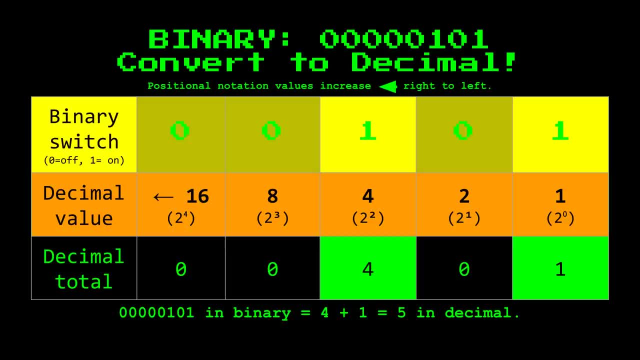 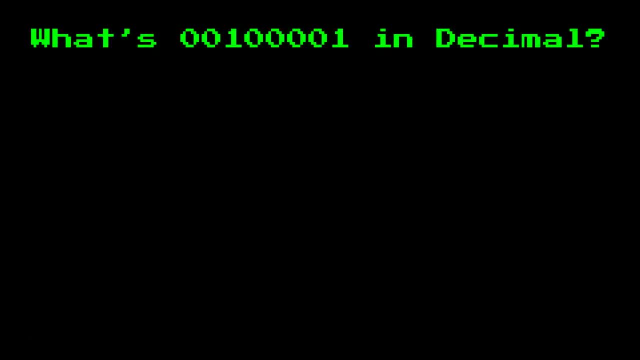 It's four plus one, It's five in decimal. You get that. It's not rocket science, It's just thinking of things in a different way. So what's a bigger number? One, zero, zero, zero, zero, one in. 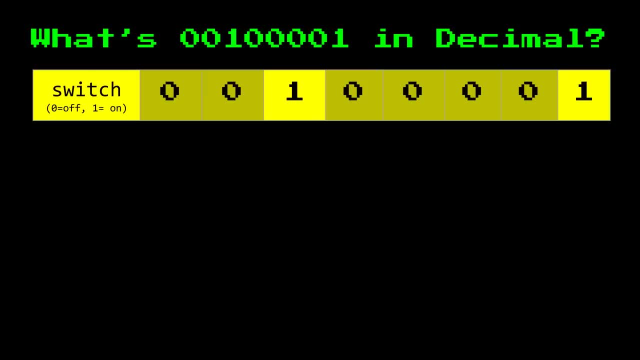 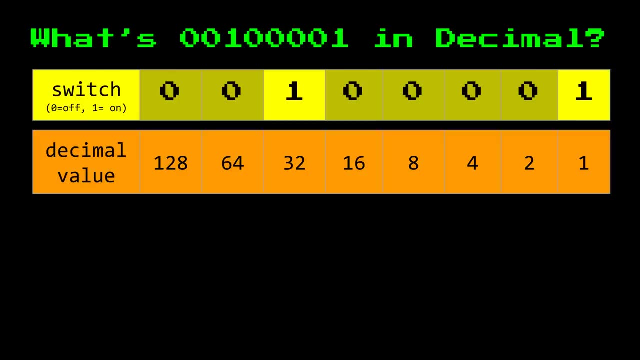 decimal. Well, switches are on in the first position all the way. remember we start to right and we go to the left, and then in the sixth position. If we take a look at that through our decimal value, we're going up to a little bit higher. now We're going up to 32.. So we see that. 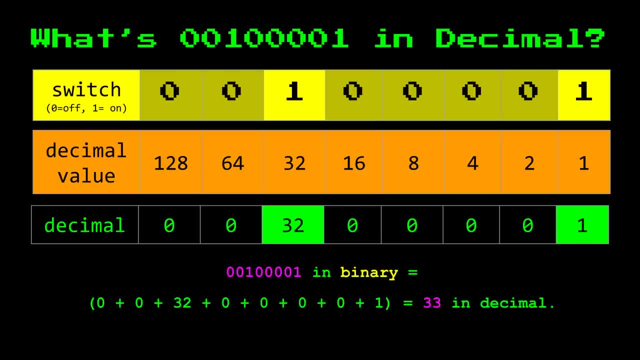 off. 16 is off. Hey, the 32 is on. So if we look at this in decimal, we can add these numbers together. So 32 is on, the one's on. We add those together, What do we get? 33.. One, zero, zero. 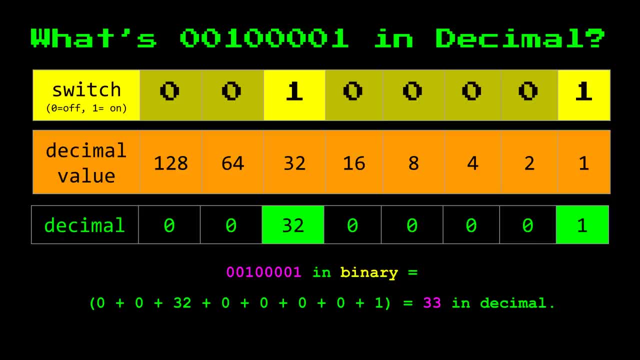 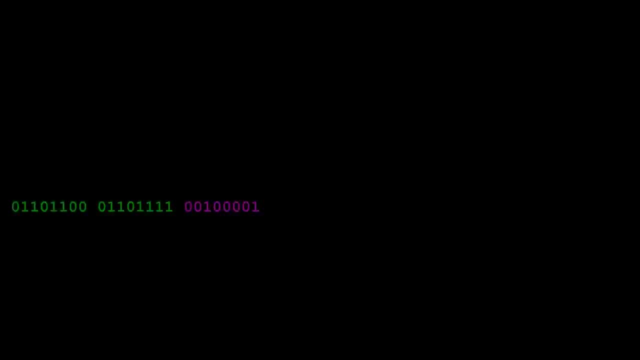 zero, zero one in decimal is 33.. Now remember this number: 33 for a second, All right One: zero, zero, zero, zero one is 33 in decimal. Now check this out. So zeros and ones might look like. 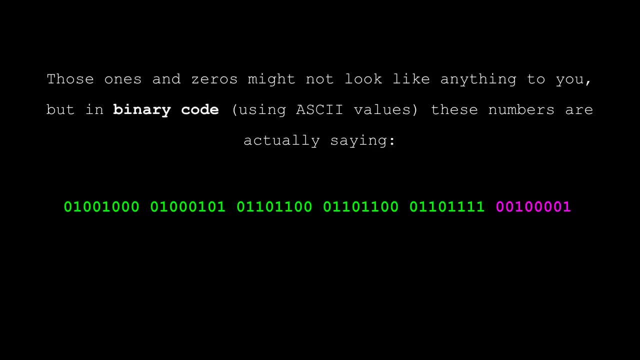 gibberish to you right, And to most people it does, until you know what you're looking at, But in binary code, using ASCII values, which is a table that translates that binary code into something else that we can understand. these numbers are actually saying: look at these numbers. Remember the one on the? 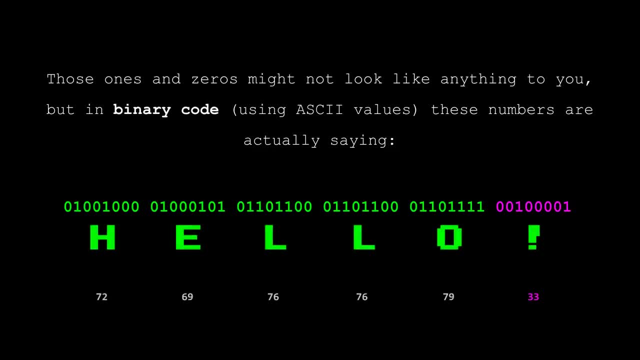 end the one zero, zero, zero, zero one. It's saying hello And those numbers underneath the letters, those are ASCII numbers 72,, 69,, 76,, 76,, 79, and 33 is the ASCII code for the exclamation. 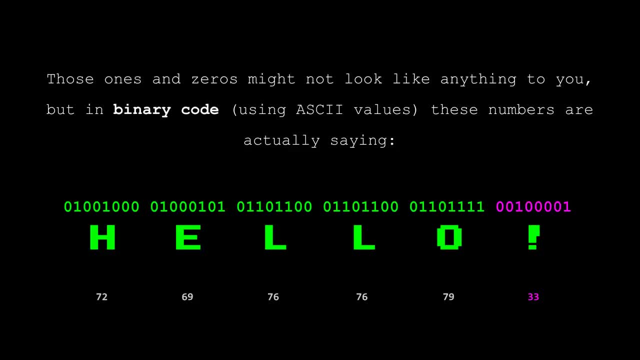 mark. Check it out Now. you won't have to remember. these computers do all these calculations for you, in binary, of course. but this is how it all works. Everything you put in the computer is converted to zeros and ones to binaries. on or off, switches to electrical impulses, to magnetic or not. Everything is code. 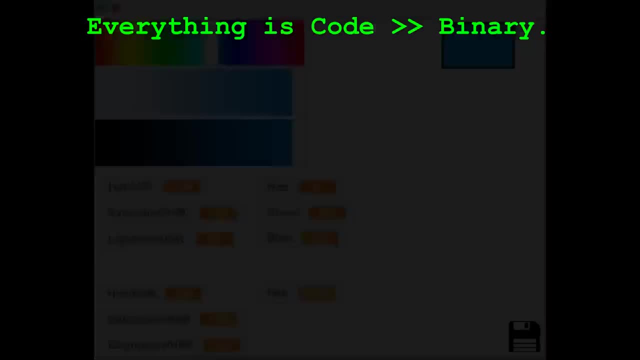 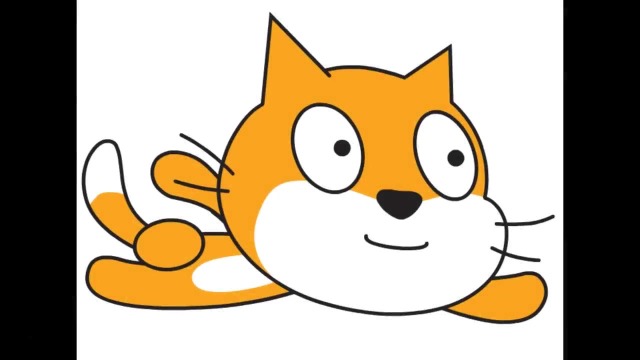 man, Everything is binary: Your colors, your shapes, your numbers, your letters, everything you put into a computer is converted to binary Pictures. every single pixel, every color, every line, every Tiny little thing, Every animation, every video, every music note, everything you do in a computer. 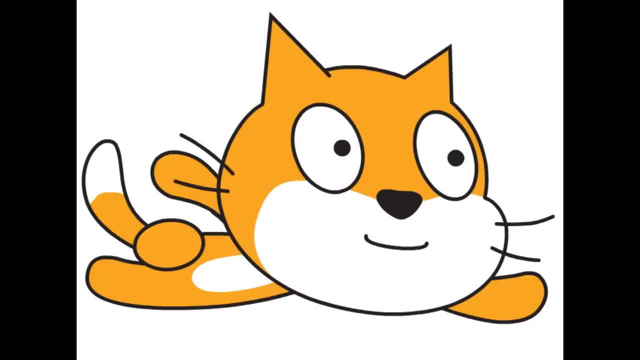 is converted to binary at some point until it can be executed by the processor. So I mean, it looks to us, it happens like in real time, so we don't even realize anything's going on under the hood. but in reality, and as we'll explain, there's so many of these calculations happening that you're 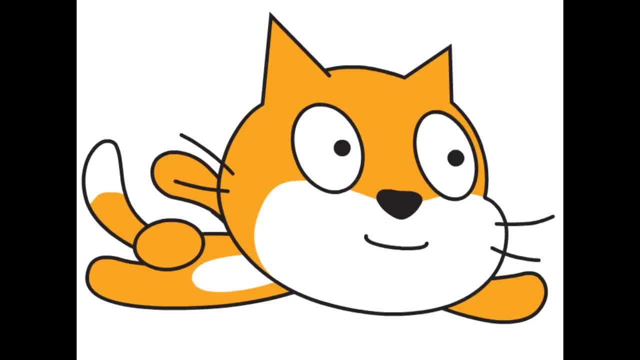 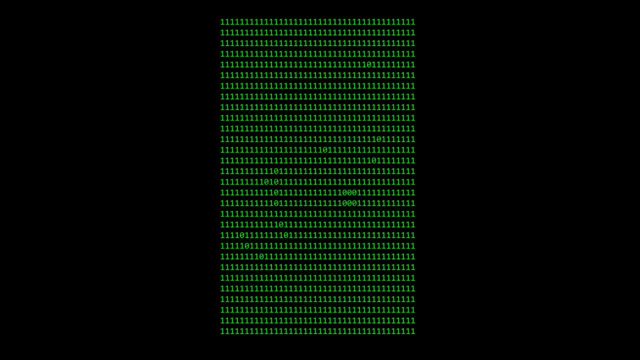 not even aware of it. It will blow your mind, but you have to understand this If you want to be a decent coder. you said you have to understand the process of it, so let's take a look at some code. right? this is, uh, that cat. 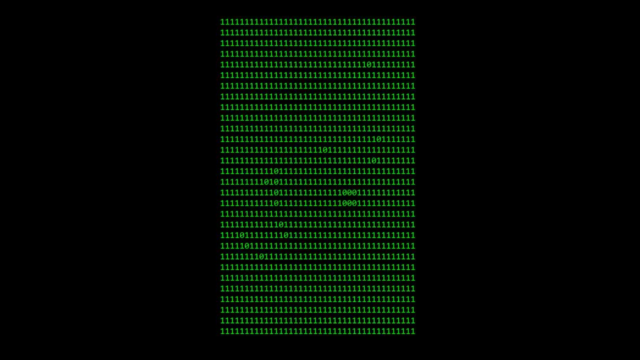 in code in black and white. this is some of the code that we regenerated by taking that picture and throwing it in the binary again, it looks like gibberish. right, remember the matrix? you saw all those green things. that's probably before your time, but all those green codes coming down, the 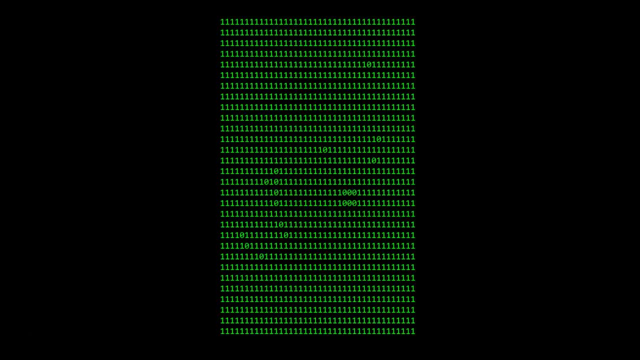 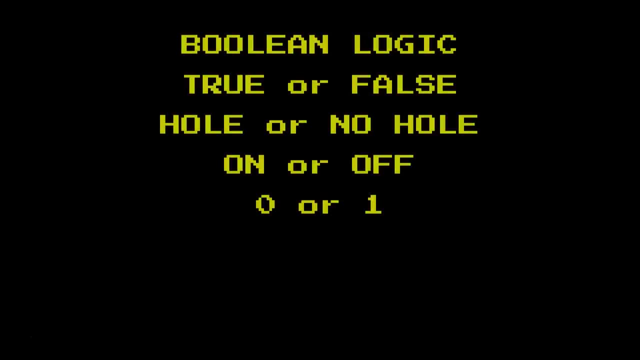 screen. that's it's code. everything is code, man. everything you do on your phone, everything you know your laptop, everything your electronic toothbrush does, it's all code. code is critical, man, it's so important we'll talk why so? we're talking boolean logic from the 1800s, true, or? 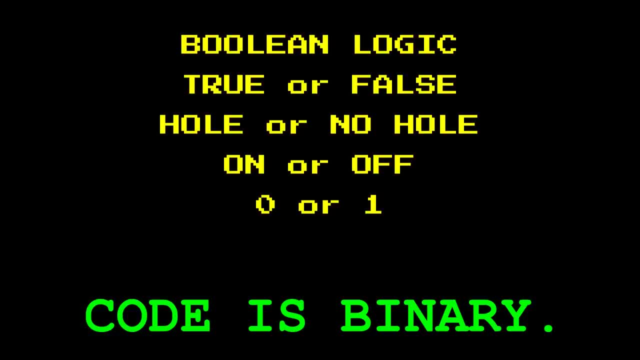 false holes or no holes, and punch cards on or off in electrical situations, zeros or one. when we go calculating the code, the most important thing to remember is code is binary on off, zero one hole or no hole, true or false. code is binary at its deepest, deepest root level. everything is zeros. 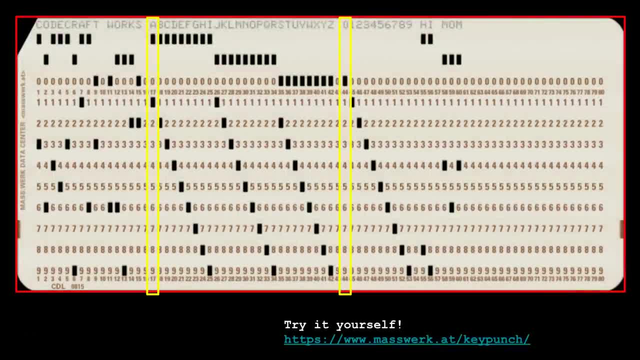 and ones, so we know that. here's a punch card. this is a more modern punch card. there's actually people still using it. these things- this is what i learned to code in back in the. i can't even tell you how old that is, but, um, people still use these. you can see that there's holes or not holes. the indication of a. 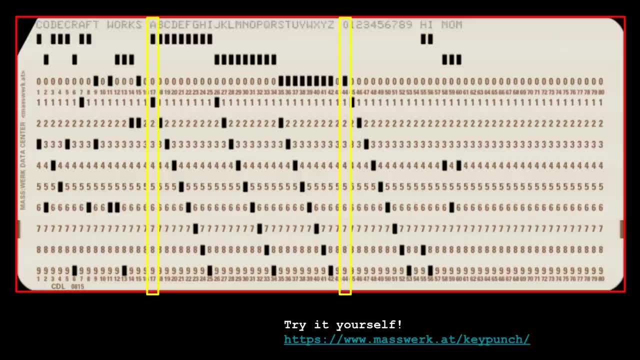 hole means it's on, no hole means it's off, and that's what a punch card did. that's what it told the early days. you needed something to feel those holes before we had electrical impulses, or a way to transmit those electrical impulses or tell if something was on or off before transistors. 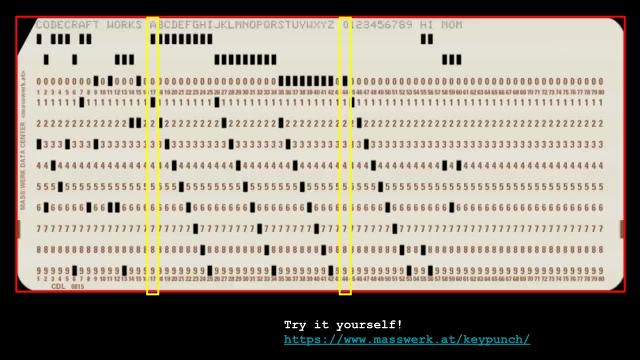 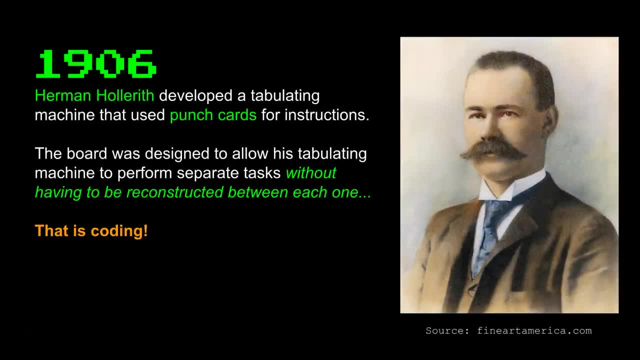 before vacuum tubes, even before magnetic tapes, we needed a way to tell computers whether something was in the on position or the off position, and, mechanically, punch cards were the way to do it. so, herman hollerith- you may have heard his names around the- uh, heard his name around the hallways of ibm. this guy's invention led to the creation of 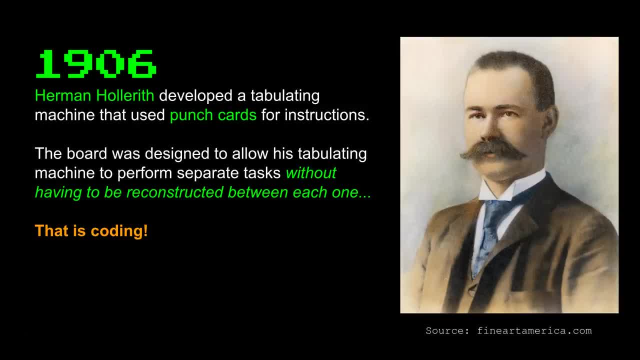 ibm, one of the biggest technology companies that has ever existed. so he developed this machine using punch cards for instructions. his code, his program, was actually on punch cards and it used binary zeros and one. so the board he created allowed his machine, his computer, to do the same thing. 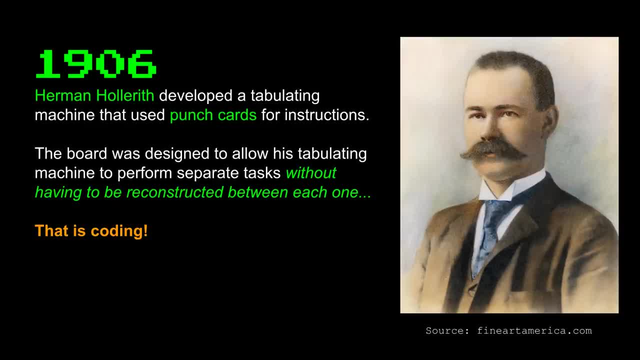 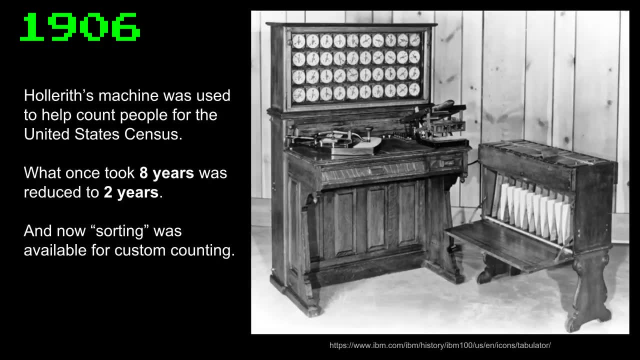 this tabulating machine to use separate, to do separate tasks without having to be reconstructed between each one. what's that? that's coding right. this is a picture of his machine from ibm's library. it was used to help count people for the united states census. you don't know what the census is. 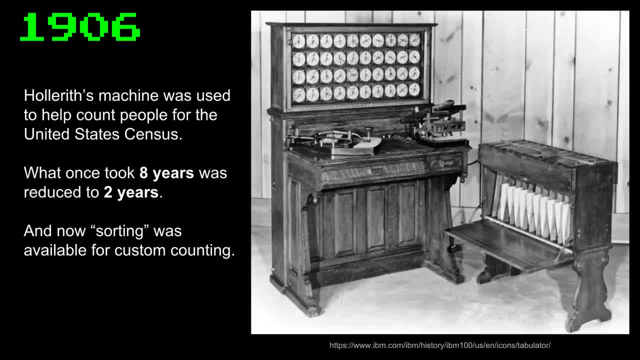 it's something the united states is legally bound to do by the constitution. we have to count how many people are in this country every 10 years, so we know how many people are here and we can figure out how many representatives to send to each state or each geographical area. we have to know how many. 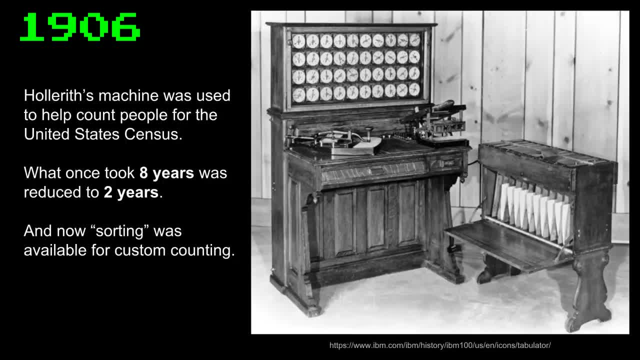 people are here, what we're all doing here and kind of how to look after ourselves. so it was kind of an ingenious thing that the the uh, the creators of our country put together and say, hey, we need to know how many people are here, so every 10 years we're tasked with counting them. the problem was it took so long to count all these. 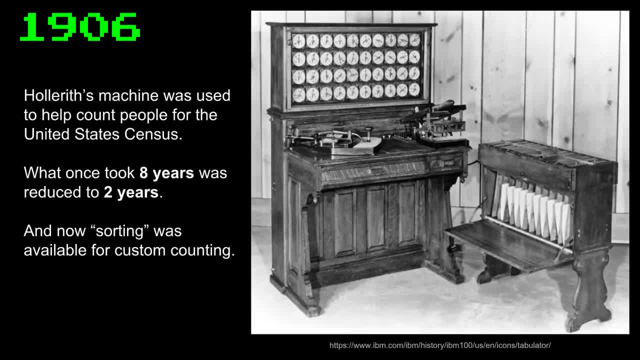 people in the 1800s, when the population was exploding, it took eight years to finish the count and by the time you had the count it was already- uh, obsolete, because they had to do it again. now, what took eight years with hollerest machine was reduced to two, and now they could. 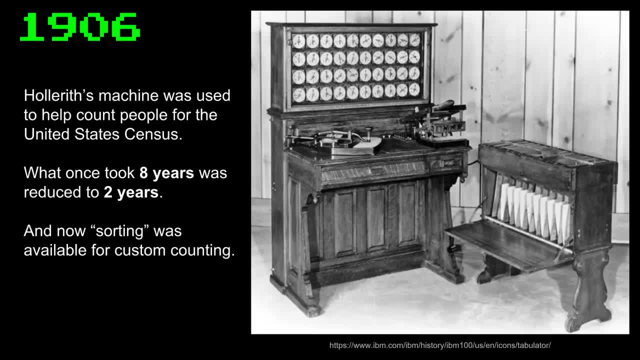 do some really cool stuff, because they could do something called sorting. never before they were able to do this. within that eight-year period, you could sort things: how many people are in a household, how many people live in this state- all from the holes in those punch cards, because each 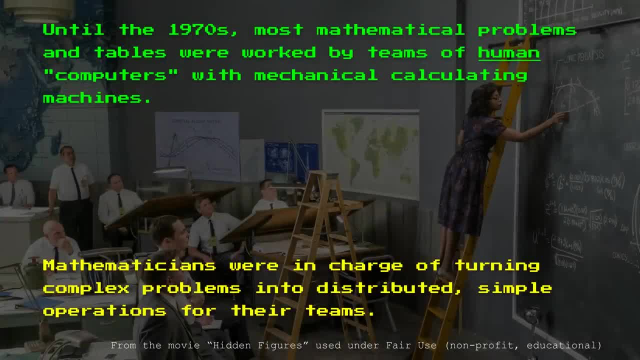 hole, had a different piece of data in it, and now we're able to do some really really cool numerical statistical calculations. now have you seen the movie hidden- uh, hidden figures? it talked about human calculators. so human computers were brilliantly responsible for computing everything, but up until then they had all these data sets. 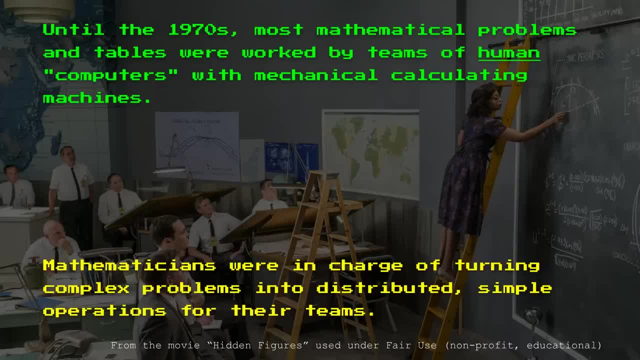 actually what they were called like rooms and rooms filled with people doing these manual calculations for trajectories for things that we needed to get people in the space and on the moon and back safe again. so teams of human computers, a lot of them were females, a lot of more women. 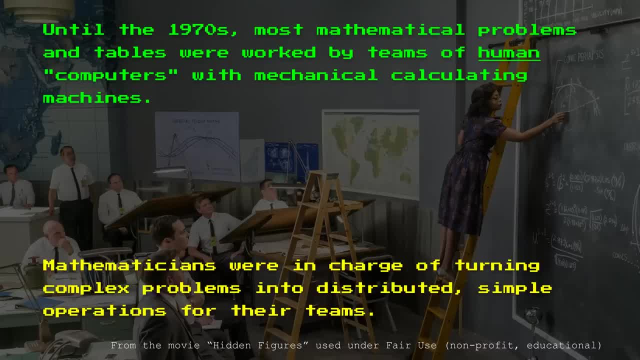 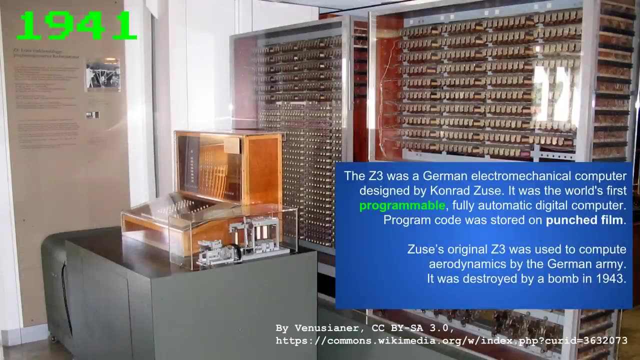 with these advanced mathematical degrees and they sit in these rooms and all they would do is calculate a small piece of a very, very complex program or a problem, and then they put it all together afterwards. and this happened even until the 1960s- 1970s, because computers didn't have the 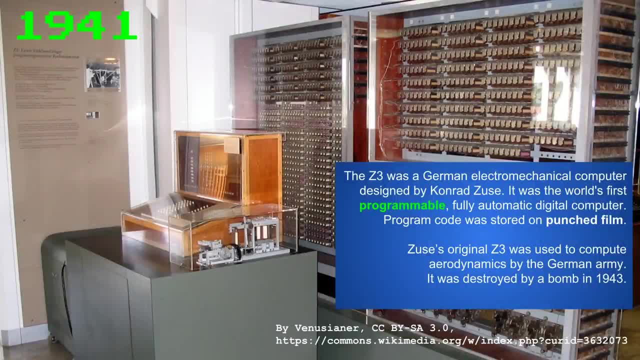 wherewithal to throw it together. so let's go back to the history of computers per se, because this will help tie it all in. so in 1941- and not a lot of people talk about this- i don't remember learning about this guy, conrad zeus, in school. supposedly in 1941, his z3 computer was the first ever. 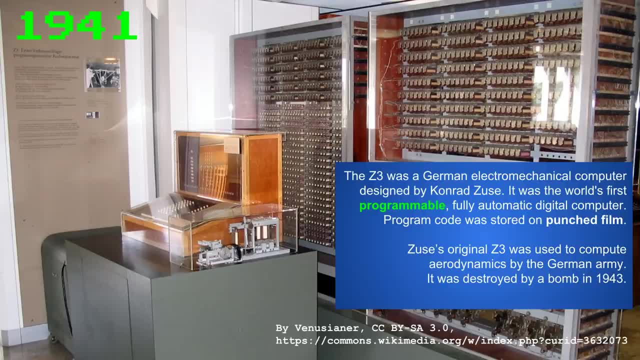 electromechanical computer designed in the world and it could actually run programs with code stored on punched film. this thing was built in germany but we had world war ii going on so we didn't know what was going on over there. and supposedly the original that was used to compute aerodynamics by the german army. 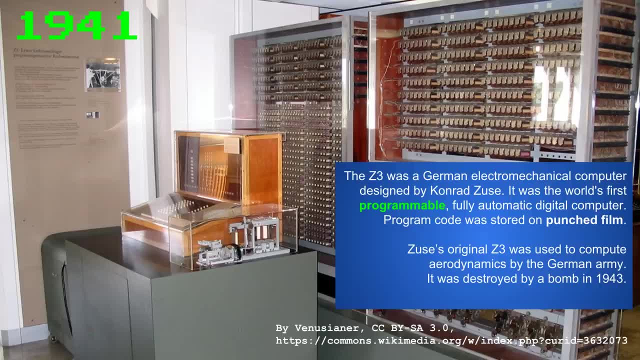 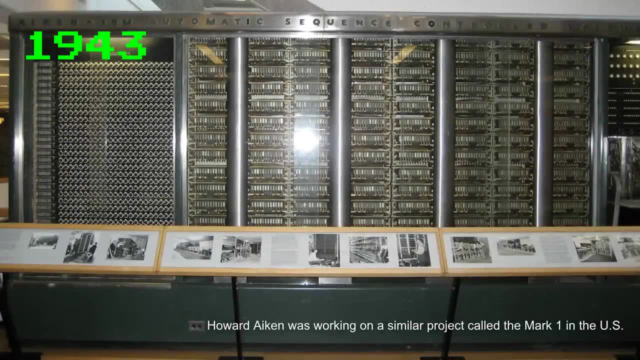 was destroyed by a bomb in 1943. so they- this is actually a replica of it, using his plans i guess they found later on- and then in 1943. so work was happening simultaneously here in the united states and supposedly due to the war, they were in the united states wasn't talking to germany because 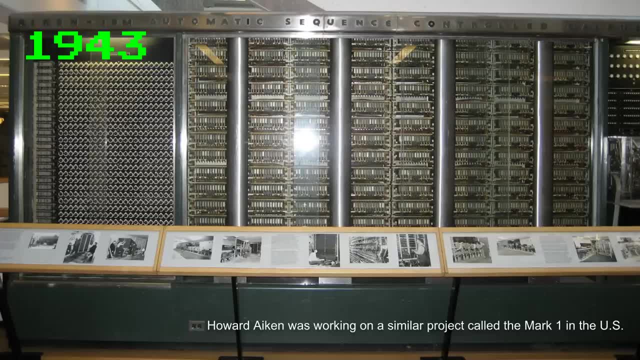 they were sworn enemies. this was happening right here in the united states at the same time. it's kind of a weird coincidence, isn't it? and this guy, howard aiken, was working on this. he's in charge of the similar project called the mark one in the united states, and look at this. 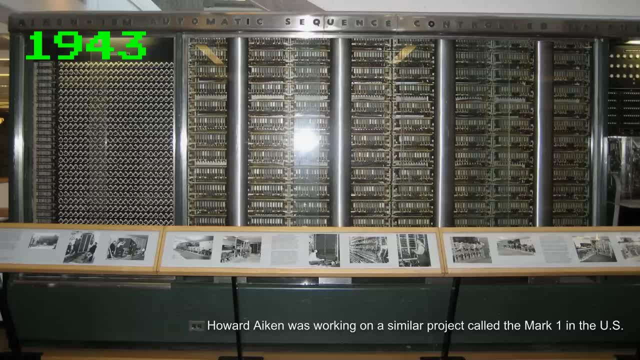 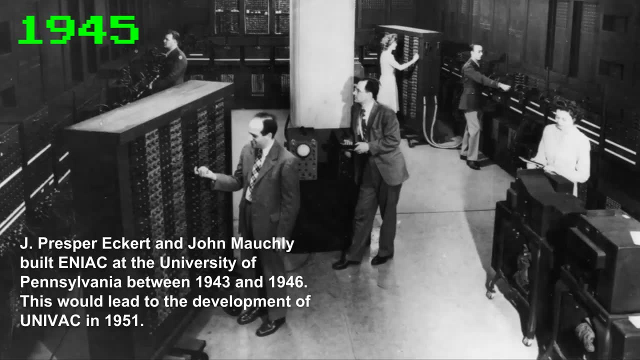 thing, man, it's a monster. and this was, uh, built by ibm back in the 40s. then, in 1945, the university of pennsylvania came up with this thing called eniac, and this is like a room-sized computer. this is where things really began to get interesting. with um electronics, we started to do things with 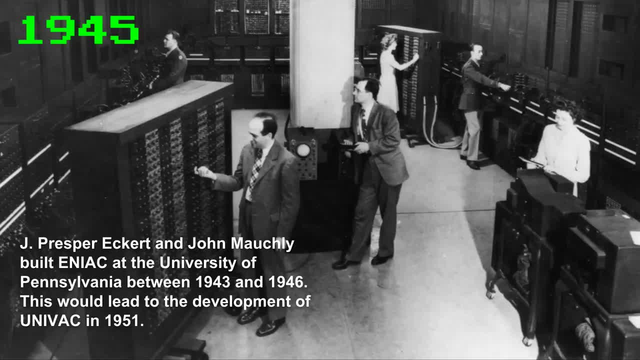 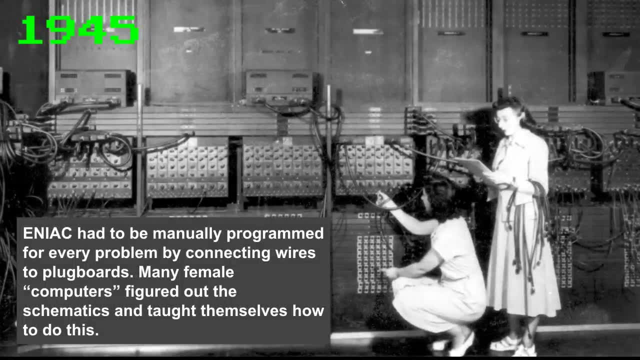 electromechanical, meaning flip switches and stuff. now we had these vacuum tubes that were truly electronic, but the room was filled with like 18 000 vacuum tubes, so it was like an easy bake oven. the thing had to be manually programmed with these wires into something called plug boards. so again, 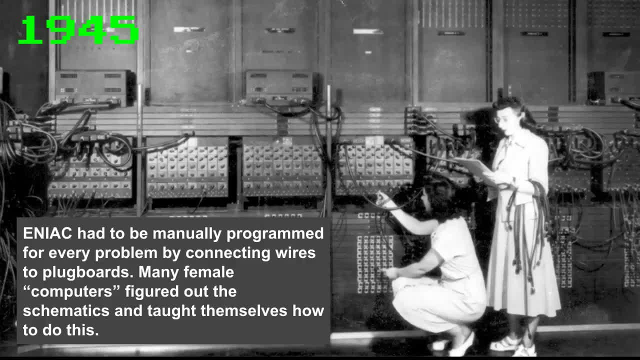 women showing their leadership in this industry. they would be responsible for number one, figuring out how this thing works, because not a lot of people knew how to figure it out and they were kind of learning as they went along. and then, number two, actually making the schematics of the programs themselves, because each one of these plugs had to be put into a 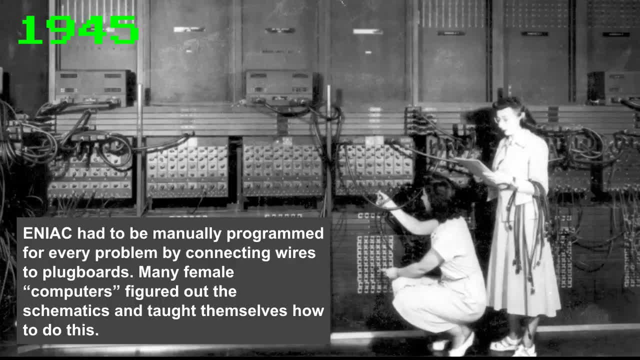 certain plug in the plug board to tell the computer which calculations to do. and every time you wanted to run a calculation you had to reset all these plugs and make sure they're in exactly the right place and then test them with a sample problem to make sure your output was. 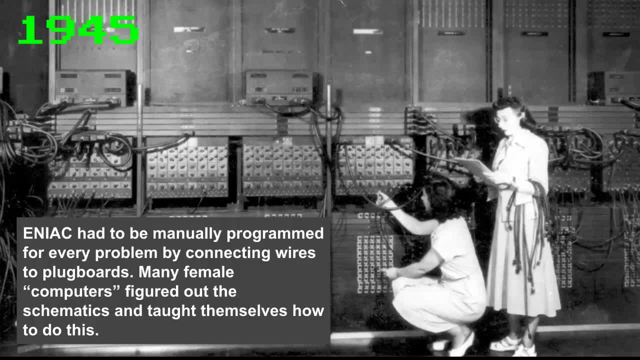 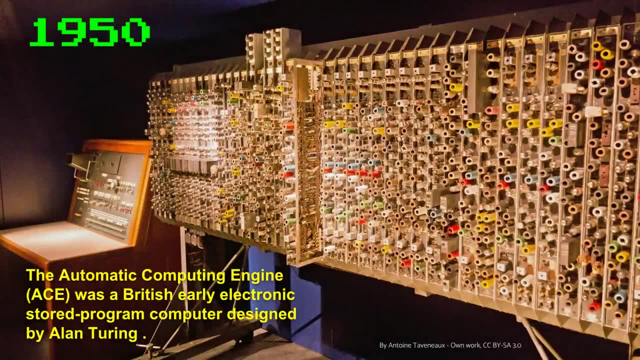 correct, and then they'd run these things for weeks and, uh man, what a crazy thing that was. i can imagine a room full filled with these things. and then in 1950, something called the ace, the automatic computing engine, was built in- uh, england, in great britain, and 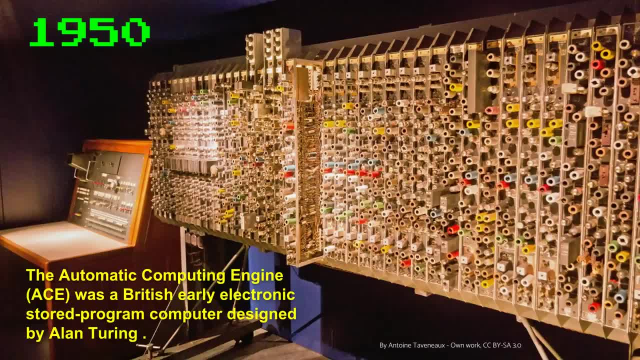 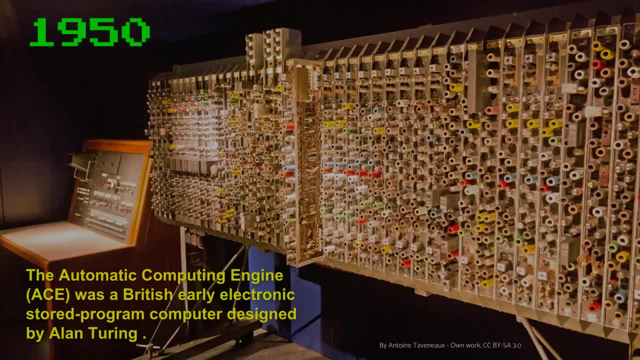 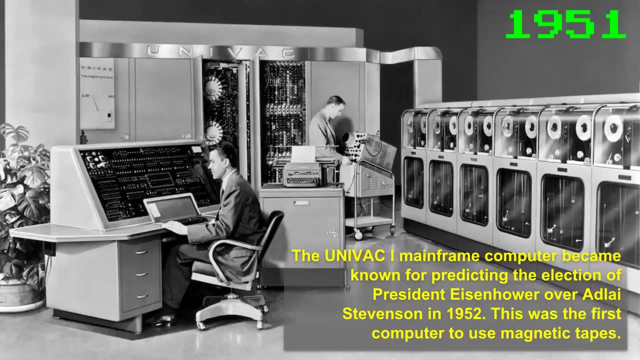 uh, it was this early electronic stored program computer with code designed by alan torren, and this was happening back in the 50s. you see, this computer and coding stuff goes way back here into the 50s. 1951 they come out with the univac and this became a big deal. this is when people started. 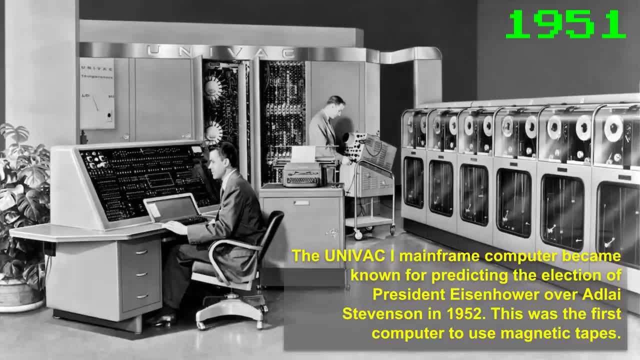 taking computers seriously, it's like, oh, i don't need one of these, they're not gonna do anything for me. but this thing, they programmed it in a way that that it was able to predict the election of 1952 in a way that people in the press couldn't. it took 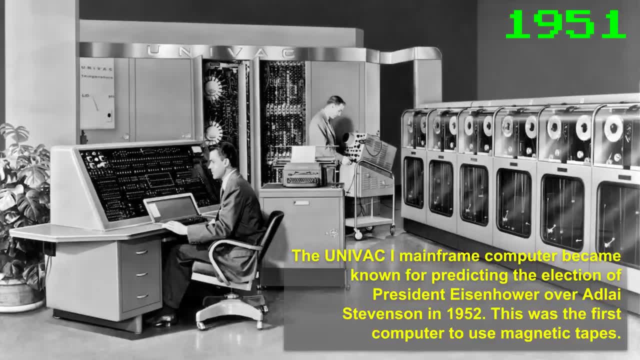 data and compiled all this data and created all these calculations that said: you know what eisenhower is going to win. and the news, people, people, news reported on this didn't believe it. they actually threw it. they're like no way man stevenson's totally going to win by a landslide. 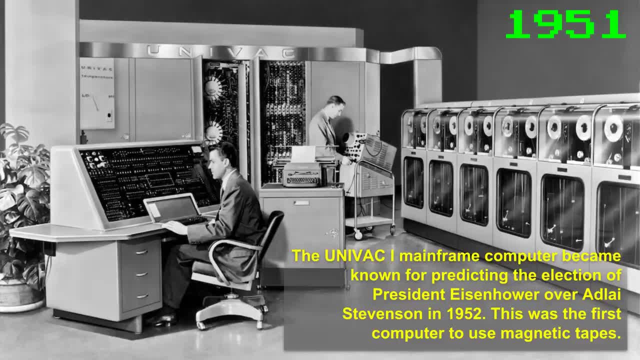 but this computer figured out this problem based on the input. it was fit, and then people started taking it seriously. this was the first computer to use magnetic tapes instead of um punch cards to store all the data. so think about that how things started to change in the 50s and then. 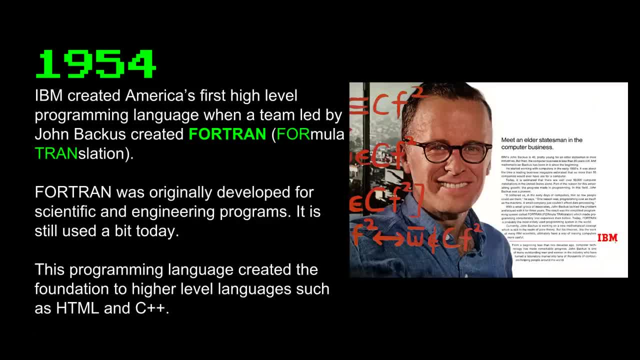 john bacchus created fortran for ibm back in 1954.. i didn't realize fortran was such an old program. it's america's first high-level programming language. supposedly the conrad zeus created one a few years before that in germany, but the first one in america that became the first commercially. 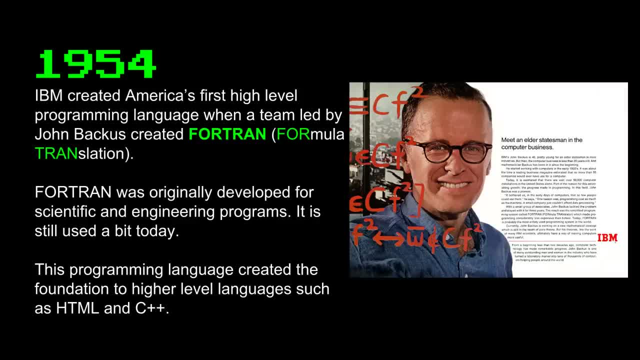 successful one was fortran. the first one in america was fortran. the first one in america was fortran by ibm, so actually used a little bit today you can make a lot of money if you know fortran. there's a lot of companies- i think mostly banks- that still have some of their systems, their 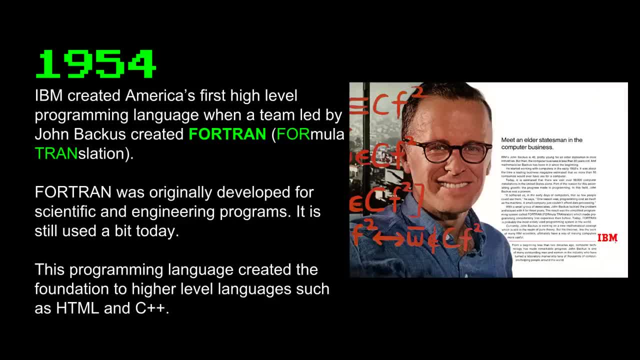 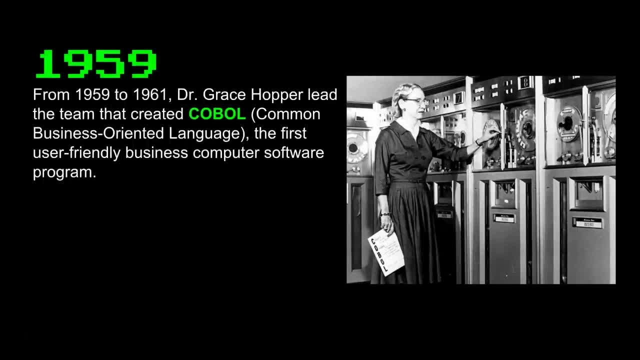 mainframes tied up in this thing and they can't afford to change them for one reason or another. so this is the basis of html and c plus plus. i'll start it with fortran, and then dr grace hopper, which a lot of people have heard of. uh led the team that created cobalt, the common business. 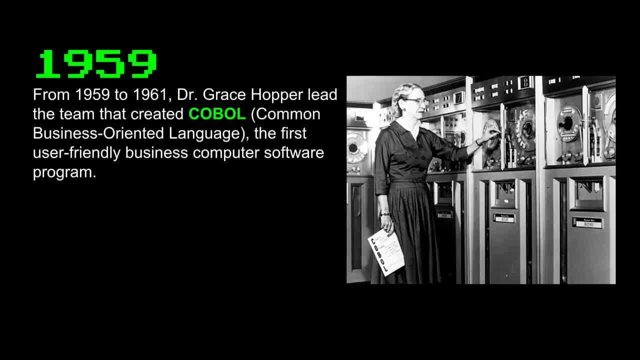 oriented language, the first supposedly user-friendly business computer software program. we learned this back in college, all the way back in the 80s and the 90s and the 90s. and also cobalt and fortran- were the two industry leaders back then- pretty similar in what they. 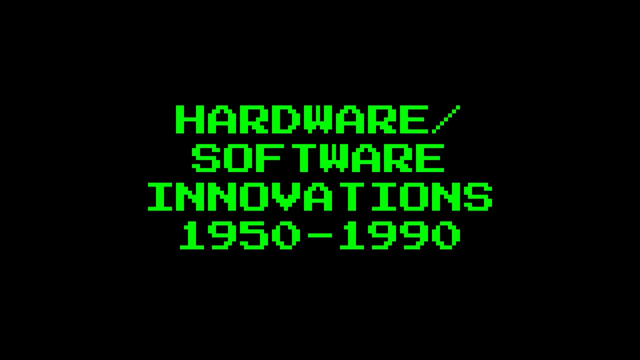 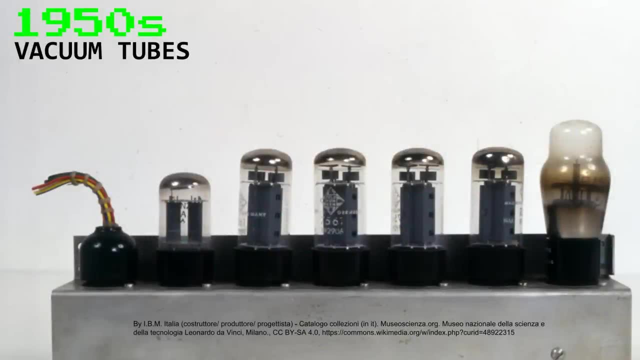 did, just a different way of getting there. so let's look at the hardware and software innovations in the 40 years from 1950 to 1990. it kind of made all this possible, so we started with these things. these are vacuum tubes, so essentially they're the these glass tubes with electronics in them. that 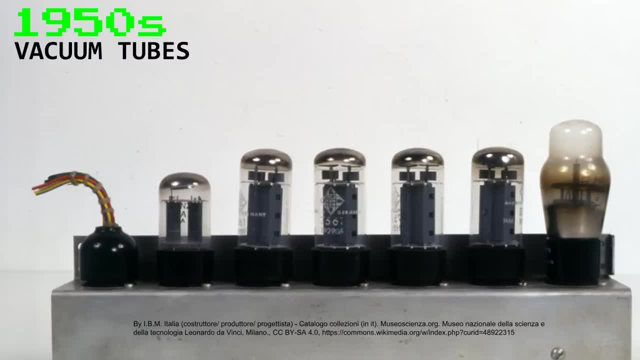 either were in an on or off position and remember some of the earliest first computers ran on these things. you had to have like eighteen thousand of them. think of these things like old and new- and you could have one of these light bulbs. they just ran really, really hot, sucked up a ton of. 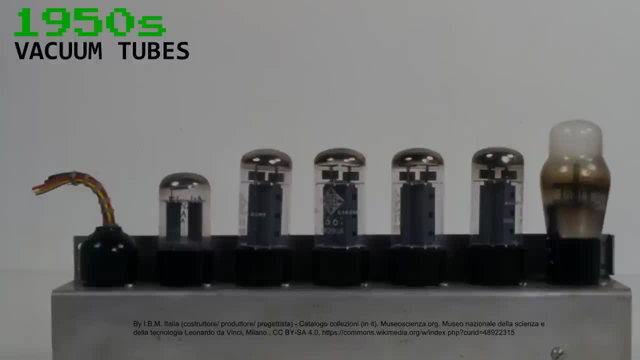 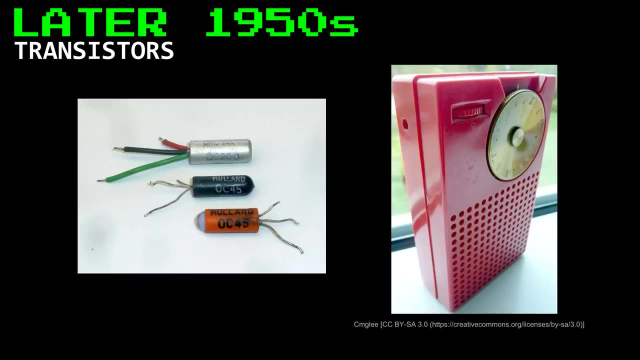 energy. it just, uh, were incredibly inefficient, but it's the only thing they had back then. and then, later in the 1950s, we came up with something called transistors. these essentially did the same thing the vacuum tubes did, except in a much smaller scale, using something called. 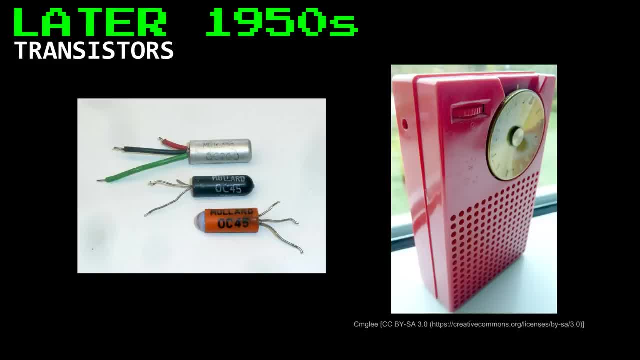 semiconductors. so we started doing this in the 1950s and then we're able- the important things- we're able to scale down the size of things. now we can make things called transistor radios, and back in the late 1950s, early 1960s this was a big deal because a radio used to be the size of a washing. 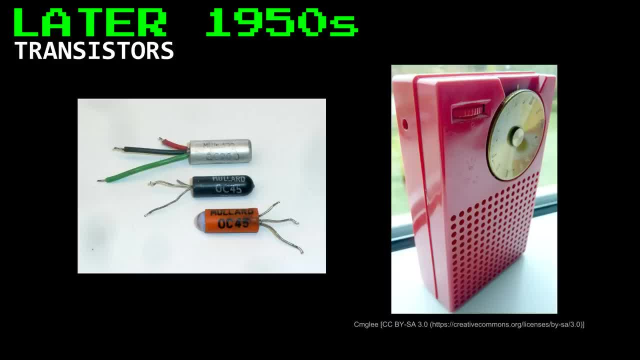 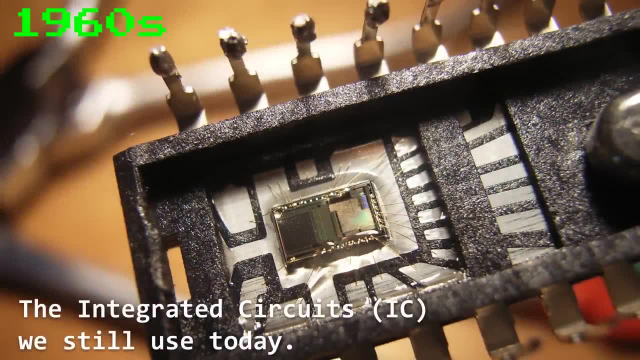 machine because of all the tubes and electronic parts in it. but now you can scale it down and actually hold a radio in your hand, and to a lot of people, to millions of people, that was just the coolest thing in the world. that just kind of took off from there. and then in the 1960s we 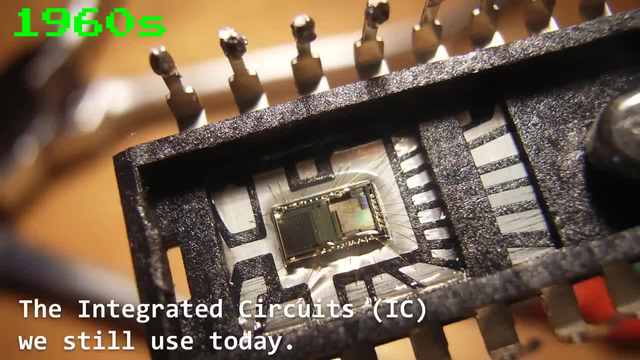 shrank, even smaller, smaller, smaller, took all those transistors and were able to link them all together on something called an integrated circuit, where other people call them chips, and this is the technology we still use today: millions and millions of tiny microscopic transistors, some. 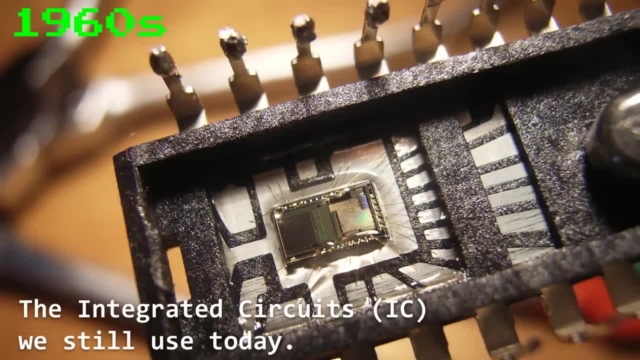 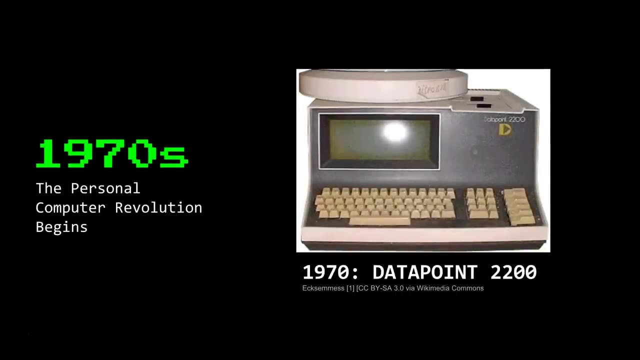 thinner than a human hair. some close the to the atomic scale. tiny, tiny transistors, on and off switches, all on this little board, that are put together to do one simple task, or execute many tasks, as we'll find out a little bit later on. so in the 1970s- hate to skip through the 60s, but uh. 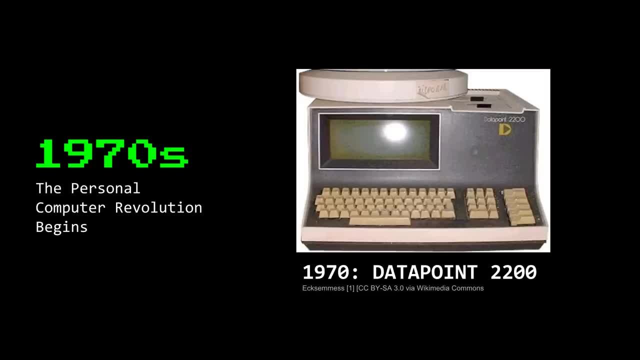 things get smaller, smaller. we're kind of working things out with coding and programming and languages and transistors and chips and all that stuff. but it wasn't until the 1970s- actually 1970, and i'd never seen this before. it's called the data point 2200, which was supposedly the first personal computer. what's? 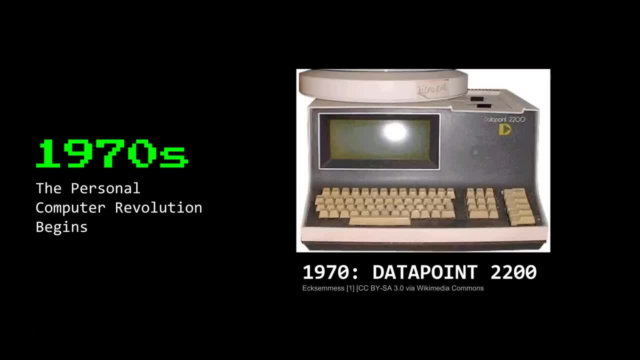 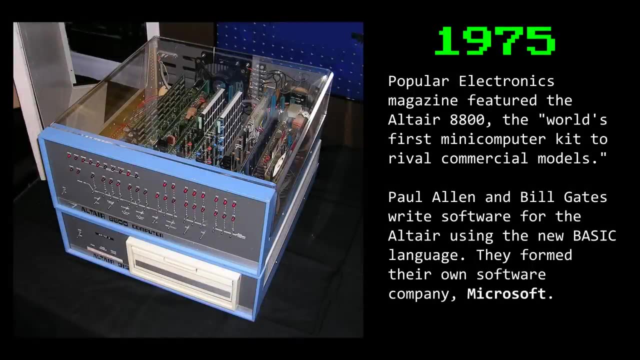 interesting about this is it had a built-in screen in 1970 and, uh, i think it's just an ibm typewriter actually throw it on there. but this is one of the first personal community may have been the first personal computer 1970.. and then in the mid-1970s, this is where it really started to take. 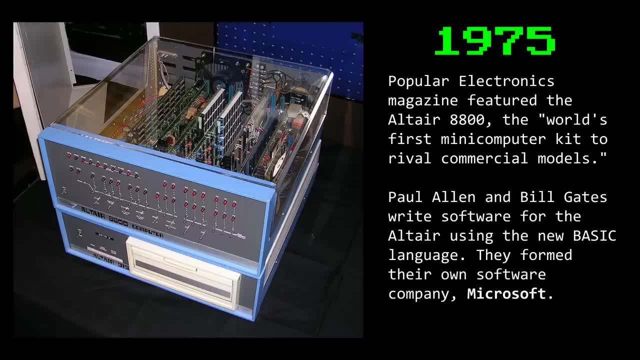 off and become more of what we recognize today. the altair 8800 was the first mini computer kit that rivaled commercial models. you were actually able to take a computer. now it was used to just financially be limited to these giant companies who have millions of dollars now. 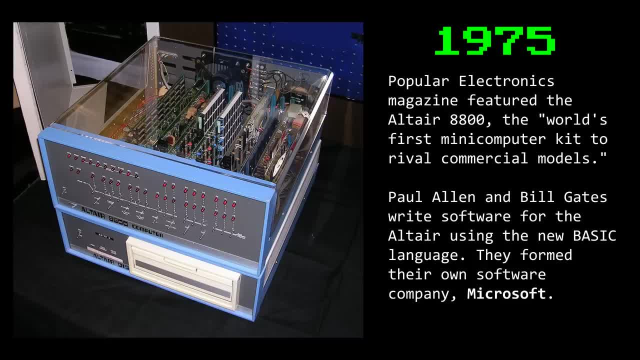 you could build something for a couple grand in your own home and bring a computer into your home. i mean, who did that? and still, they're a bunch of naysayers, you know. say, oh, you'll never need a computer. what are you gonna need one of those for? 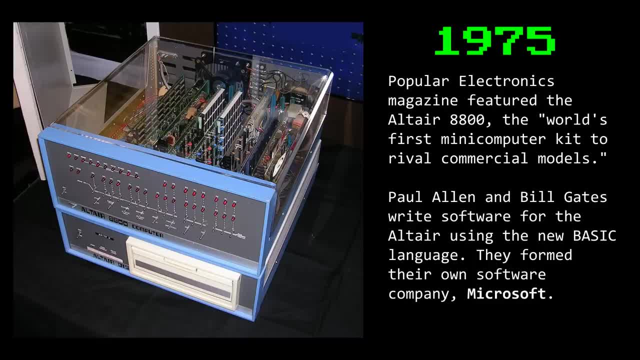 paul allen and bill gates. you may have heard of them and they wrote some software for the altar using the new basic language and they formed their own company called microsoft back in 1975.. hard to believe it was that far back right. this thing didn't do much, did simple calculations, but 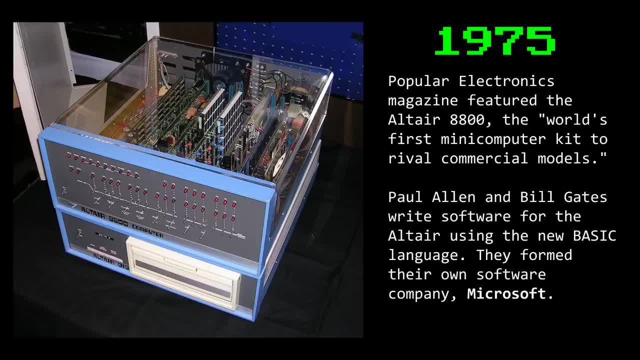 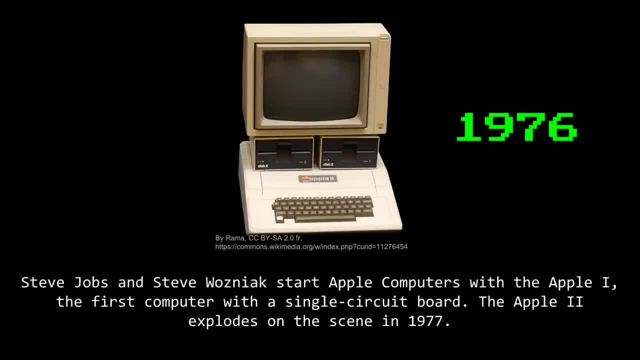 people were able to uh actually with the development, since they were able to do some games and some really creative things with this thing. this is really where it started to explode in 76. steve jobs, steve wozniak, you know, these guys started apple computers with the apple one. 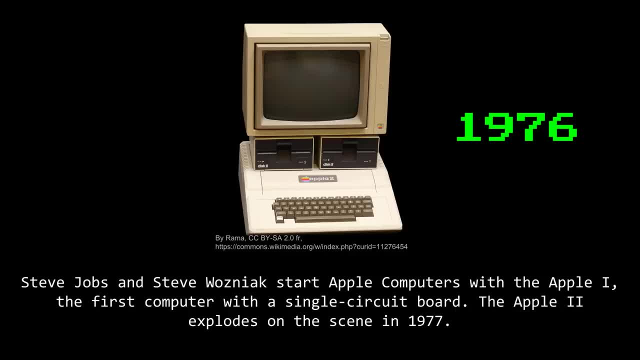 and it was the first computer with a single circuit board. then the apple ii in 1977 and then this is the first computer i ever remember seeing, first personal computer. i ever remember seeing, after coming off of teletypes and punch cars, man, but i was like, wow, this is amazing technology. 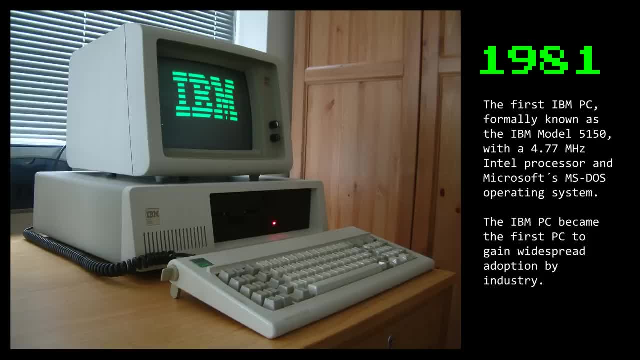 1981- 1980s was when ibm started to take off and make these things smaller, more affordable and actually functional enough that they appeared in almost every professional office. this was the first pc to gain widespread adoption by the industry: a 4.77 megahertz processor, not gigahertz, using microsoft's ms. 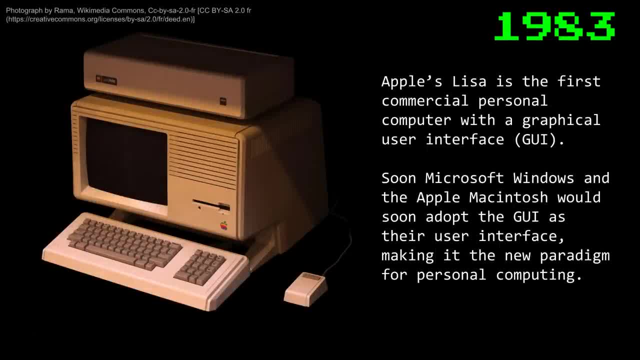 dos, and this is really where microsoft began to take off too. in the 1980s, apple's lisa comes out with the first graphical user interface. they call it a gui, and this is where you see the little mouse move around the screen and you can click on icons instead of typing in words. 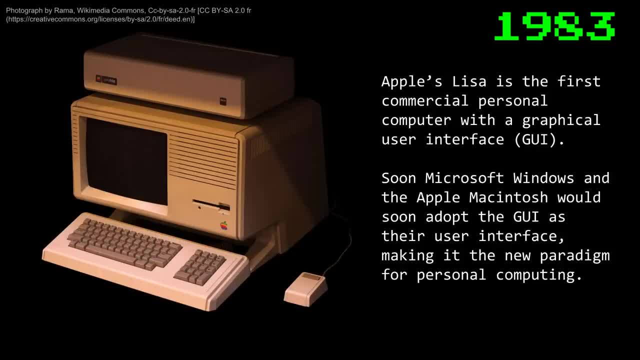 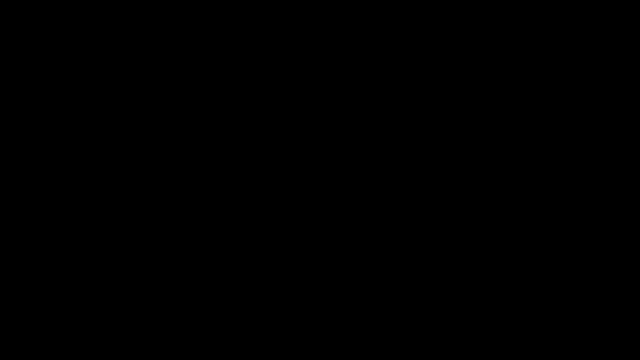 so soon microsoft, windows and the macintosh would adopt the gui, and that's kind of what we use today. imagine typing things on the screen to do your programs. it's got to be uh kooky, right people- coders- still do it. so there was a. 1984 was a big year for the personal computer: apple, macintosh. 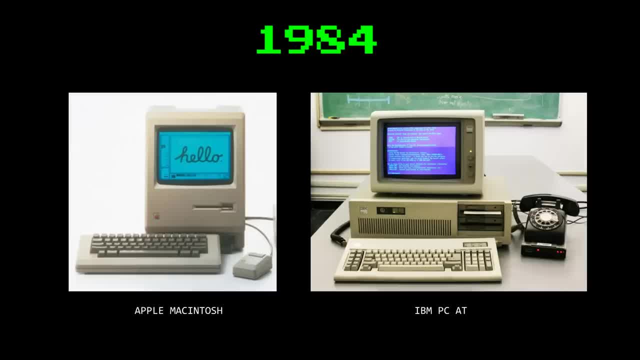 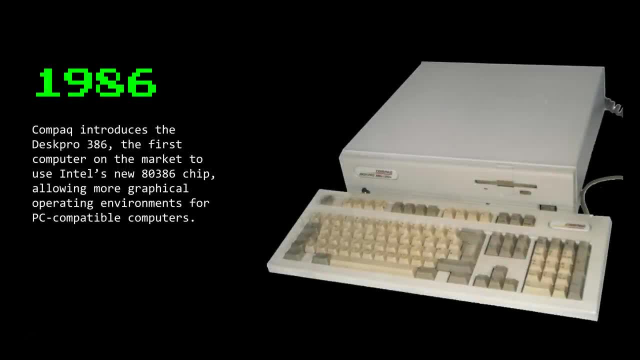 came out in the ibm pc at and uh color displays and see that thing on the right. that's called a modem. that's how we used to connect to other computers. we'll chat about that a little bit later. pro 386: now this was a big deal. i remember hearing about this like: whoa, you got a 386 before. 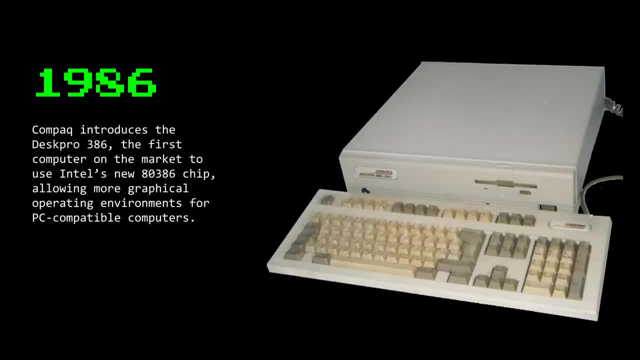 that was a 286 which was really slow, sluggish. with the 386 man you could do some really cool graphical stuff with this computer. this was actually my first business computer, a 386 computer, when i was working for an insurance company man. it was just the coolest thing in. 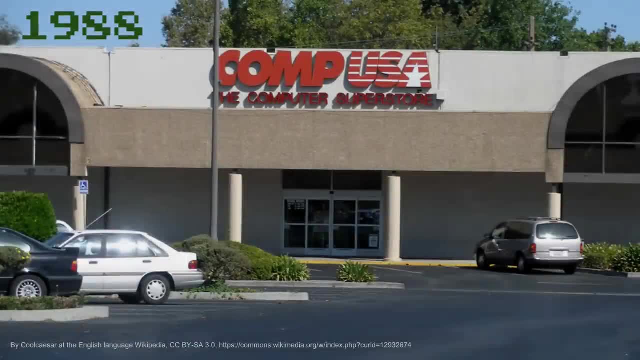 the world with what you could do on the screen, with these things, with spreadsheets and word processing- things you couldn't do before then, in 1988, man. this is when the industry really began to explode and you started seeing stores like comp usa pop up and 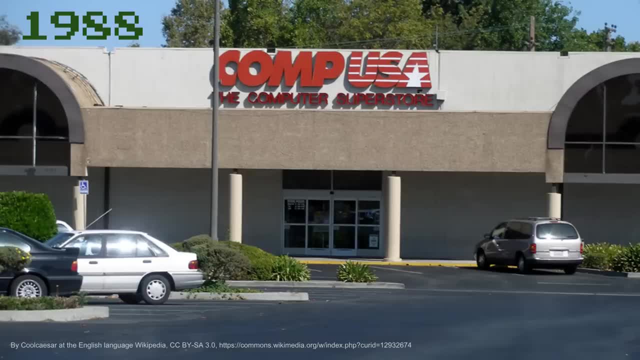 the gateway country. stores and computers, just stores filled with computers and games and peripherals and monitors, and oh, the smell of plastic in that place was just unbelievable. this was the coolest thing that ever happened in my life. i used to hang out in these stores. i just go to the store. i couldn't afford a lot of stuff in there but i just go and just. 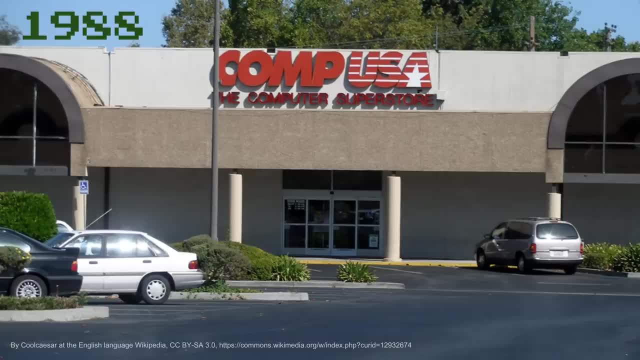 every couple of weeks, just be amazed at all the new technology that came up. so yeah, i used to hang out in these stores even until the- uh- 1990s, till they went away. they just broke my heart when they disappeared. i hope they come back. i mean fat chance. but 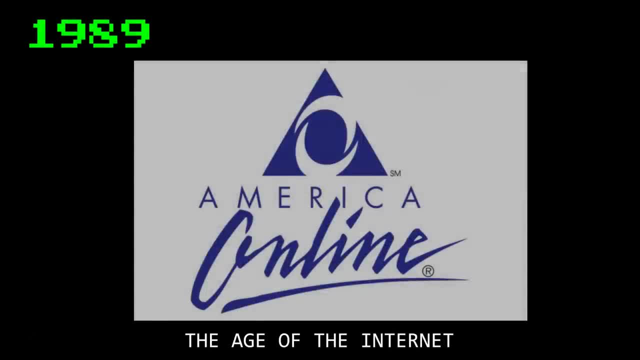 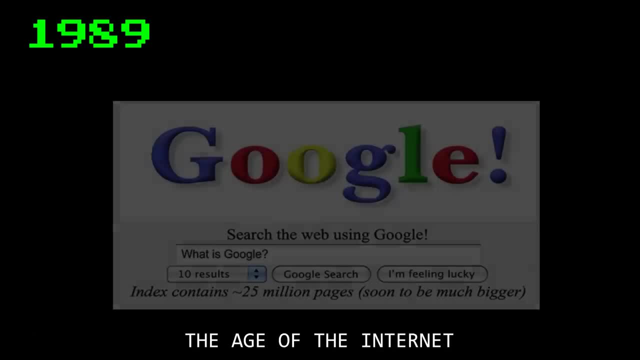 probably not with the internet. and then in 1989, the 90s, the age of the internet, you saw aol jump on the scene and then lose it to broadband. you saw yahoo become the king, lose it to google. amazon's still here and, uh, google's now kind of king of the industry. we saw my face. 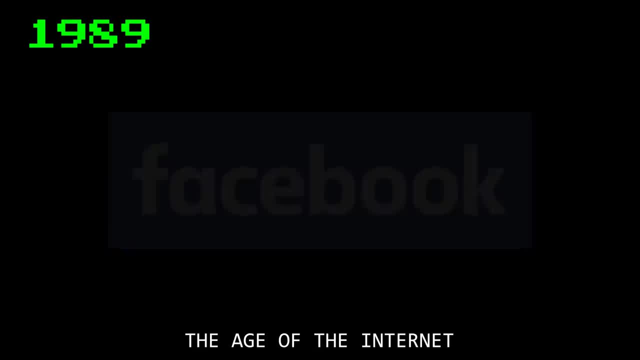 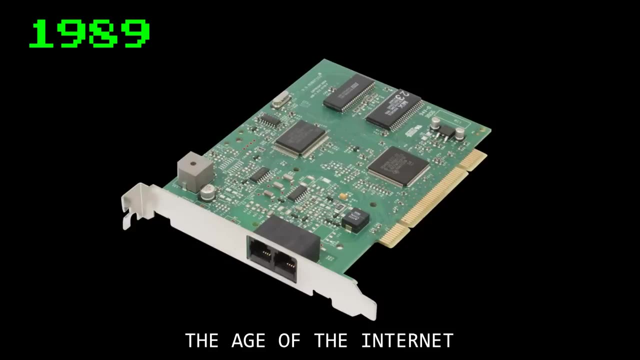 get eclipsed by facebook. a lot of changes. what you usually saw was the. the pioneers usually didn't make the cut. they had a great run, they made millions of dollars, but then a number two, a more nimble competitor, took over and did things a little bit better. 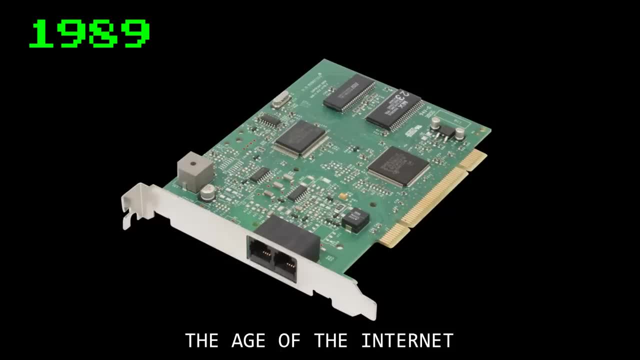 think blockbuster, then netflix think yahoo, and then google think aol, and then all these broadband providers think: you know it's just. and then the modem. this is how people used to connect to the internet back in the early days over. it's called pots, plain old telephone service or plain old. 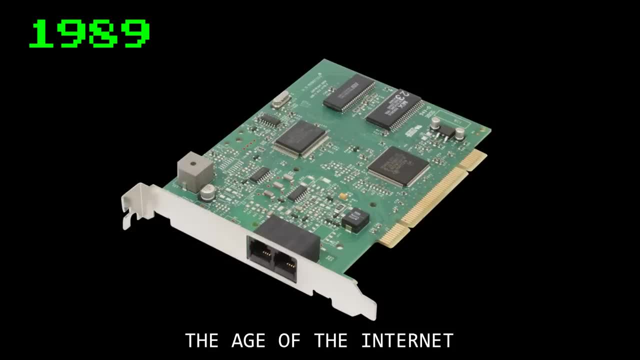 telephone lines. it was painfully slow. 56k was as fast as you could go and they had some compression algorithms made a little bit faster, but really not much. it wasn't really made for streaming video until broadband became mainstream, that your cable companies and your phone companies started. 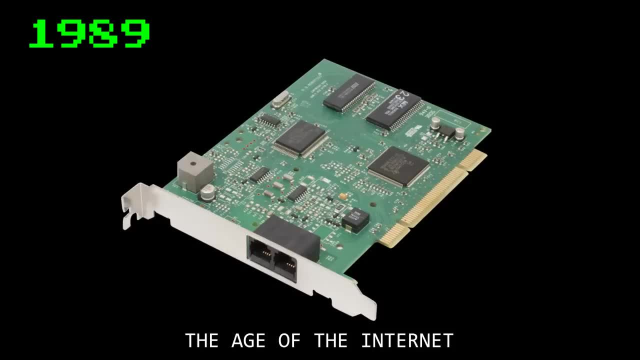 offering dsl, and that's what really made the internet take off. but the fact that you could send an email to somebody around the world without putting a stamp on it and you didn't have to wait for it to get there- it was there like in seconds- was the coolest thing in the world. i still remember. 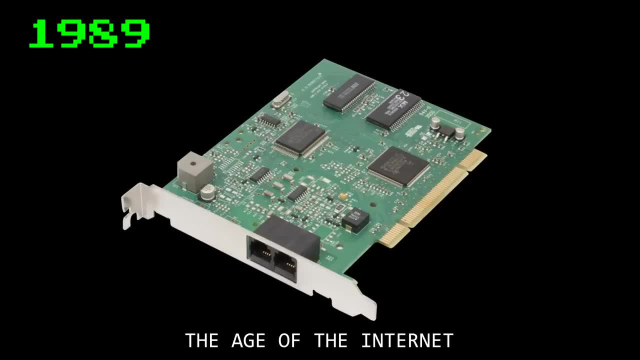 it just blew my mind, opened up a whole lot of opportunity for a lot of people who wouldn't have had those opportunities, including myself, including my first book deal, my first magazine article. so the age of the internet. and then, once the internet became uh, everywhere everybody had. 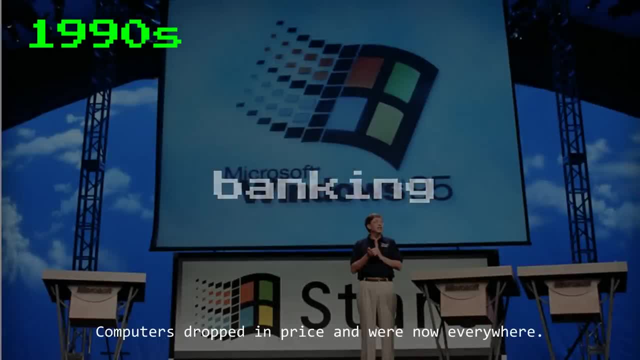 to have these things. but now these computers. in the 1990s you could do banking, you could play games on them. computers were dropping the price. you could do shopping. you never had to leave your house anymore. email people were using this for customer service, for everything computers were. 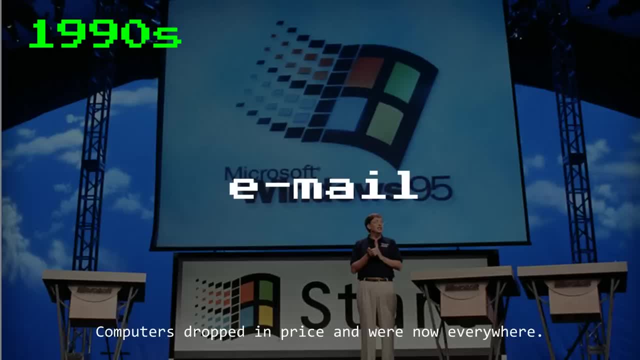 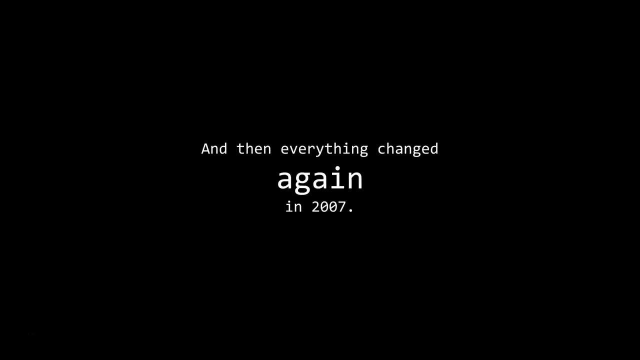 being used to do stuff and they were still kind of pricey back in the day. but the prices were dropping and there's getting more and more adaptation and, uh, it really blew up into the early 2000s until about, well, 2007 and everything changed again. you know what happened in 2007. this: 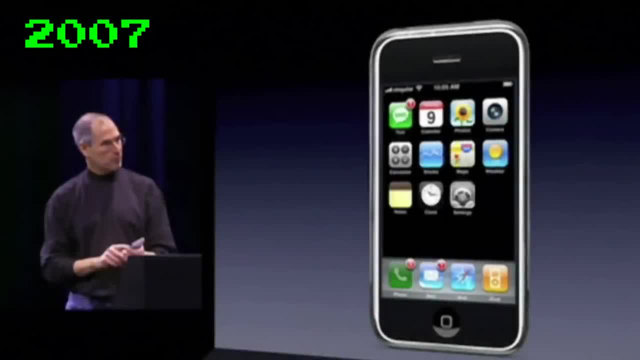 guy, steve jobs, said: let's come out with something called a smart phone. now we had the technology to basically do almost everything we could do with a computer and put it in your pocket. you're no longer stuck in one place, having to plug something in. now you had this battery operated device, device that would last most of the day. 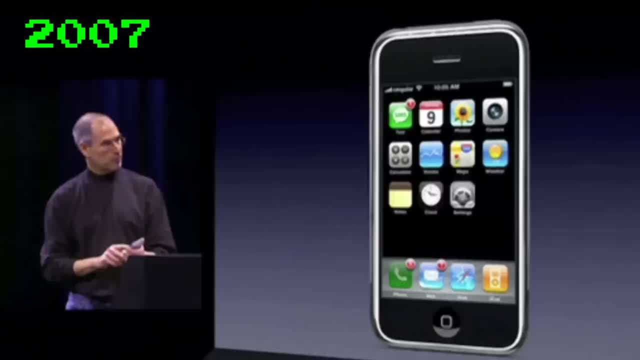 now you could send emails on it, you could, um, check your stocks, you could check the weather, you could, uh, play games, basically everything you could do on your computer or your laptop. but you're kind of. you're kind of had your hands tied because you had to be in kind of a, a stationary location. 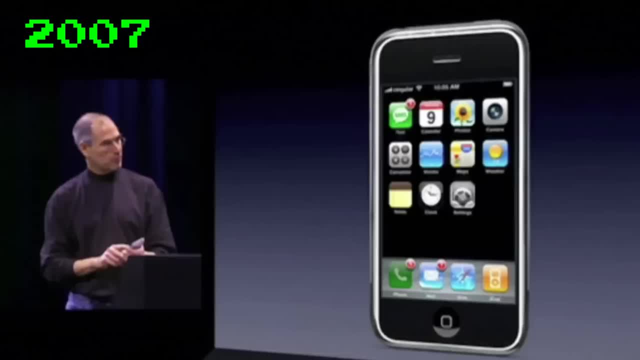 now. you could do this on the go, you could do it on a bus, you could do it on a train or playing in an airport doctor's office while you're waiting. i had one of the first iphones in brevard county. i saw this coming and i owned a computer repair facility back in the day. 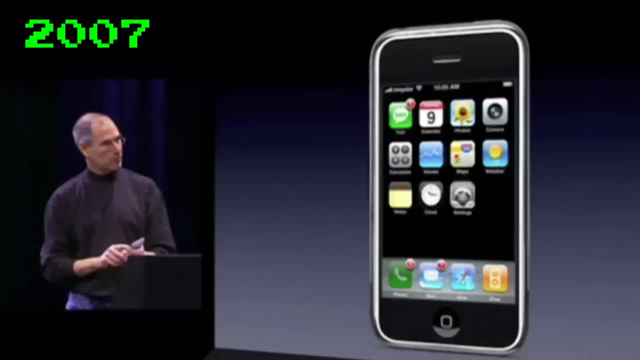 and i saw this in 2007. i said this is the end of us, it's just a few years, because you couldn't repair these things. i mean, you could repair them, but you really didn't repair them. you replaced them every year or so and uh, you know a lot of computer businesses, kind of. 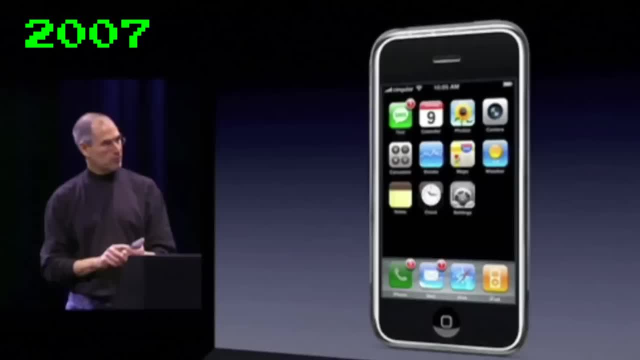 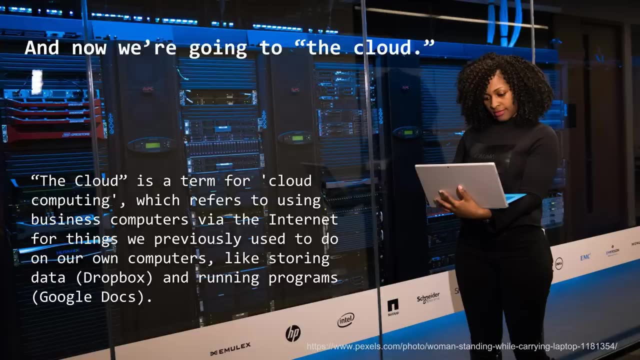 faded and folded because of this technology, but it's still, to me is the coolest thing in the world. and they got faster and faster and smaller and smaller, and now you're seeing a fundamental change where people are are no longer storing things on their computer, they're storing their 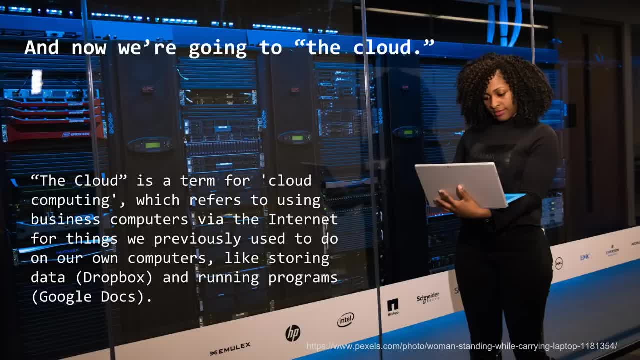 pictures, storing their documents, storing their videos in the cloud. and what is the cloud? people ask me. is it actually a cloud? no, it's not a cloud. we just think of it that way, because it goes somewhere and it's up there and we need to worry about it no more because it's a cloud, just go with. 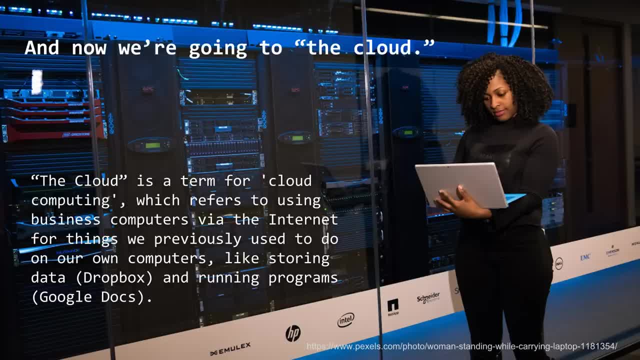 the cloud. it's actually a great term. you think about it. clouds are up there, they have their little function and uh, they're there one day. they're, they're, they're, they're, they're, they're, they're. well, they're not, then that's a problem. but the cloud is essentially a bank of computers. 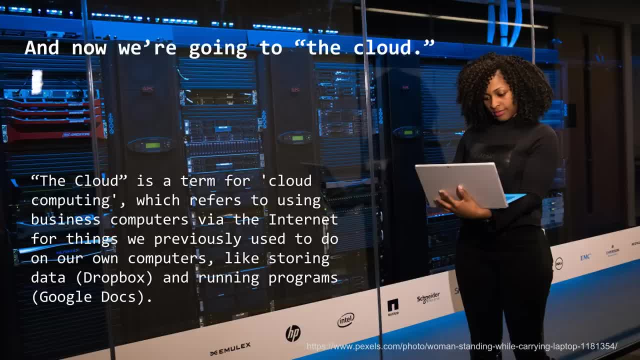 think of it like a network of computers maintained usually by a large company, with redundant backups all over the country, even all over the world, is story or stuff, and it's pretty darn reliable too. and now applications like google docs. i have a lot of kids that have never run microsoft word. they've 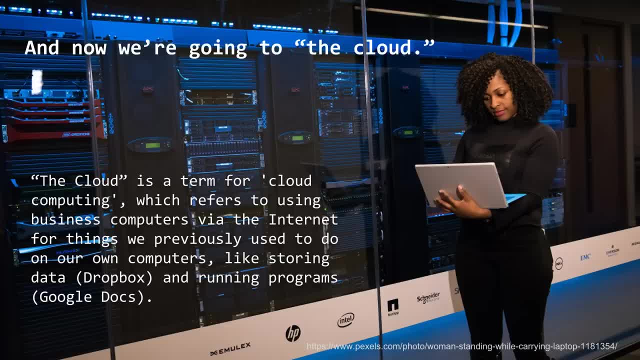 always used google docs because it's in the cloud, it's free for most people. why spend a subscription? does basically everything. office does. this slide deck's running on google docs, so your documents, your pictures, your data is being stored on the cloud. applications are moving to the cloud too, so we went from smart computers to we actually went from dumb terminals. that 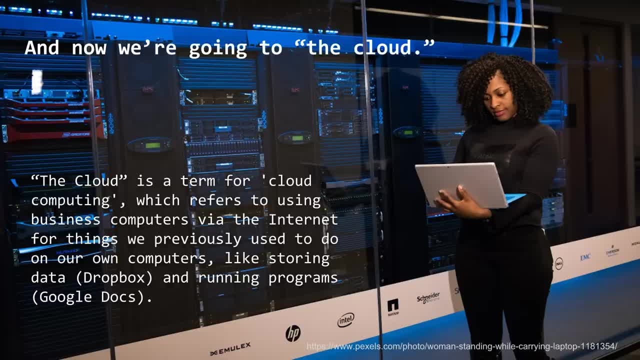 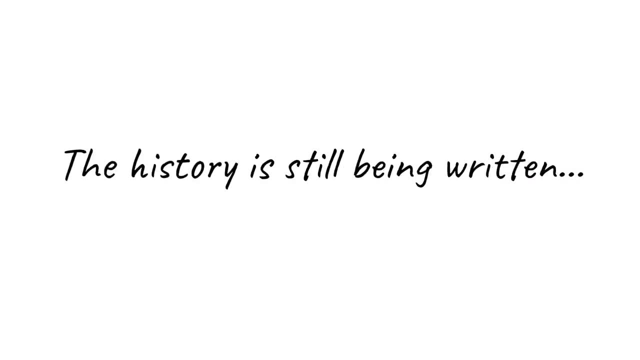 were centralized like this, running on a local cloud, to smart computers that didn't need a cloud. and now we're back to the cloud again. so it's funny how these things are cyclical. the history is still being written, ladies and gentlemen. every day, a change comes up, a. 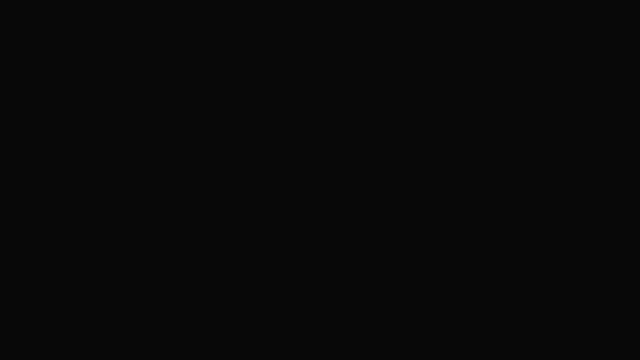 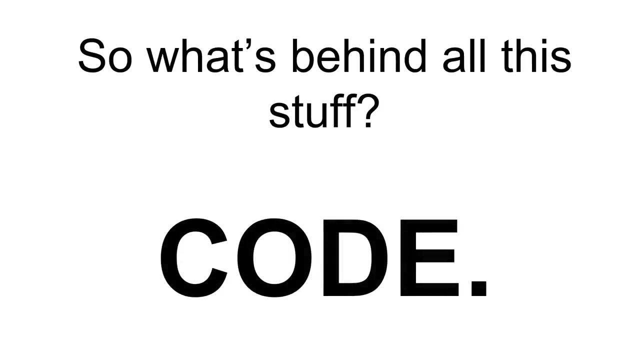 new electronics and technology industry that's going to change the world tomorrow and make it completely different than anything we know. so what's behind all this stuff? we go back to code zeros and ones binary. what is coding? well, look on the left. it's- uh, this kind of weird. 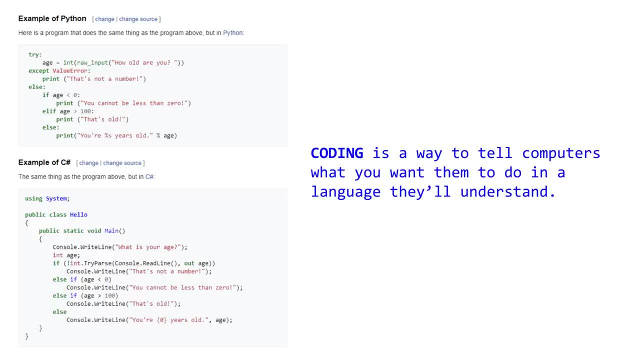 combination of words. it's a way to tell computers what you want them to do in a language they'll understand. basically again, computers are stupid. they don't know what to do until you Explicitly tell them what to do in a language They understand. that language is binary. 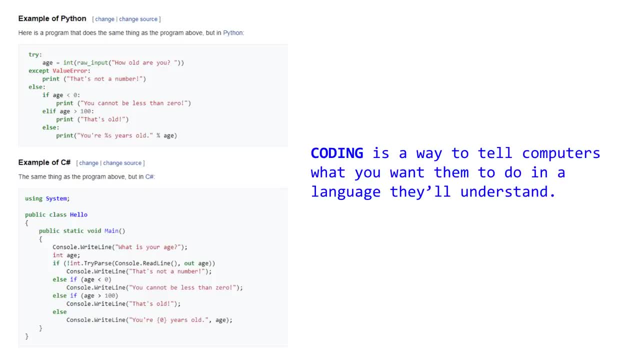 But the way to get there is you have to use some kind of code which will then be translated into binary. So we had to set up a set of rules. All right, if we write these Words in a certain way, in a certain order, then we can convert that to binary and the computer will know what to do. 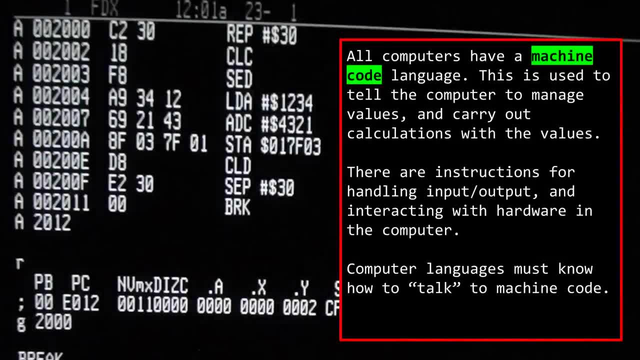 We call that coding, So all computers have this thing called machine code. It's kind of like a real, real low-level language Used to tell computers how to manage values, carry carry out calculations, where to store things in memory- Essentially, instructions for the computer with what to do with the hardware in the computer, and all computer languages must know. 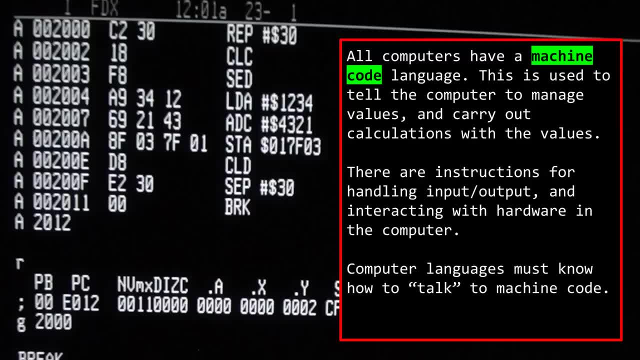 At their lowest level, how to talk to this machine code and translate everything to binary. This is where it all ends up, and some people could actually program games and applications in machine code. Supposedly, this is the most efficient way to do it, But it's the most difficult way to do it too. 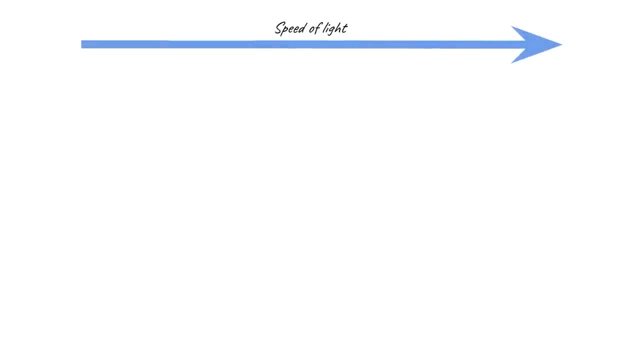 Very few people do this. So what happens with a computer program with some code? what happens? What? the speed of light will nearly the speed of light. speed of light in a vacuum. Anyway, it was pretty darn close. So you take your top level language or your lower level language, whatever you use, create your code in your favorite language. 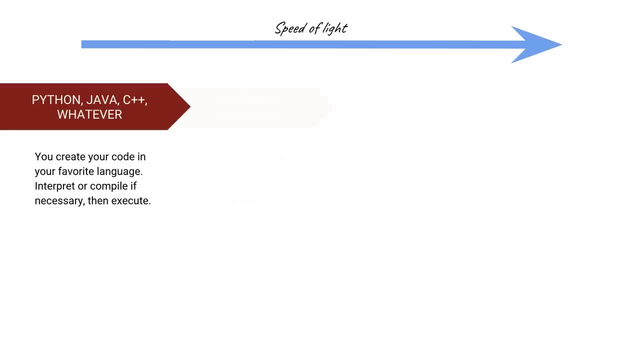 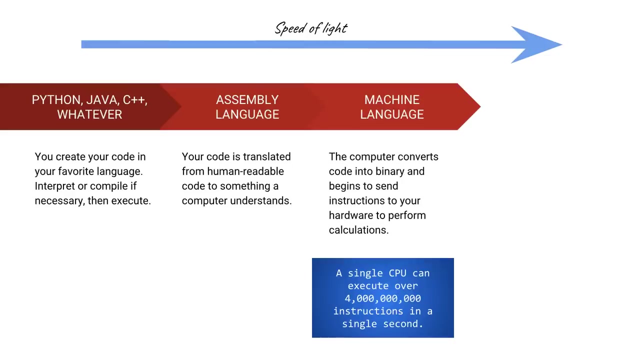 And then you're gonna interpret or compile it- We'll talk about that if necessary- and then execute it. So then in some cases it shoots it to something called assembly language. right, It takes a human readable code, puts it into an intermediate intermediary. Another language is something a computer understands, and then your computer translates that into machine language. 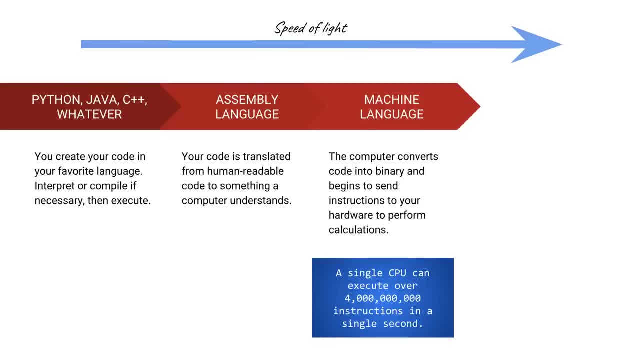 it begins to send those instructions in machine language through your processor and your memory and to your video card to perform those calculations. and a single modern CPU can execute over four billion instructions in a single second. think about that number for a minute: four billion instructions or calculations, or 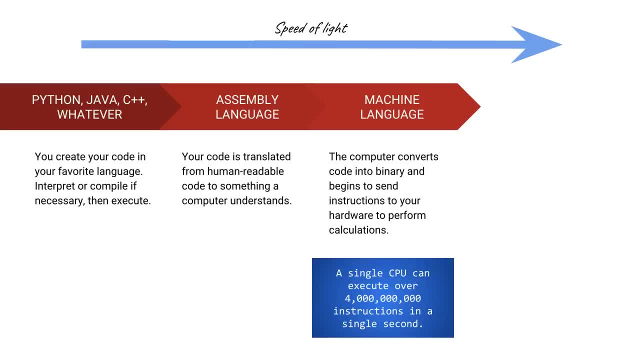 or whatever in a single second. that's just mind-blowing that it could happen that fast and be done so well and perfectly almost all the time. it's just mind-blowing. it's got to be alien logic right. and then when we have that machine language, it sends it to. 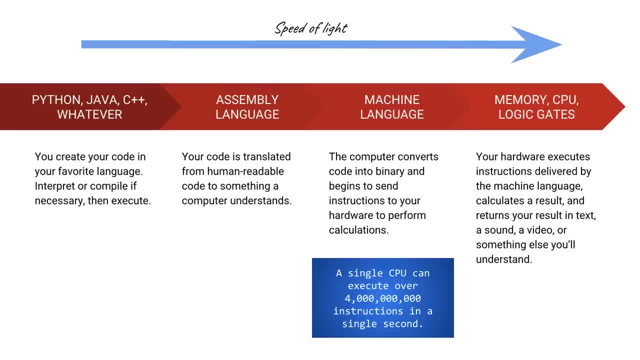 your computer, you remember your cpu, logic gates and your hardware does all this stuff. and then it returns a result again in something that you as a human can understand: a picture, a word, a sound, whatever it was, a result on a calculation, whatever you told it to do through that code. 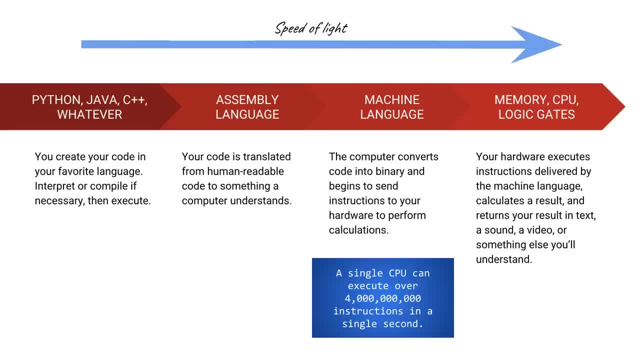 or whatever you told the code to do, or whatever the coder told the code to do, and then you put your data input in there, whatever you understand what i'm talking about. but basically it's doing whatever the code tells it to do and then returns a result automatically at the speed of light based. 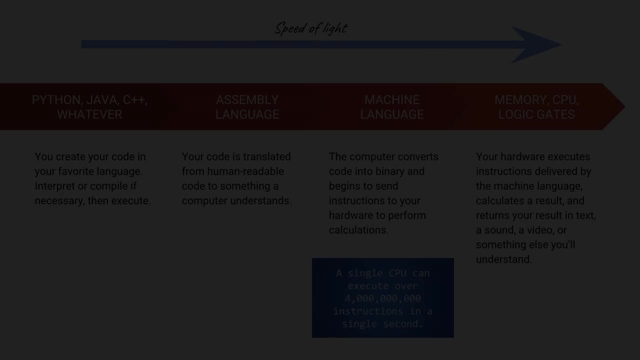 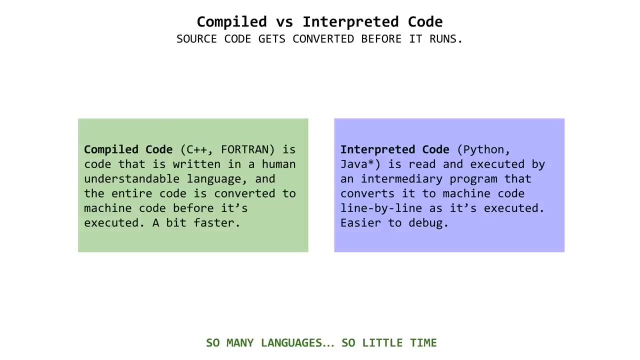 on that input that you threw in your computer. it's hard to think of. but uh, let's dig a little deeper. so we have something called compile code. so we write code in like c or fortran in a human understandable language, and the whole code is converted to machine code before executed. so a lot of people think this is more efficient because 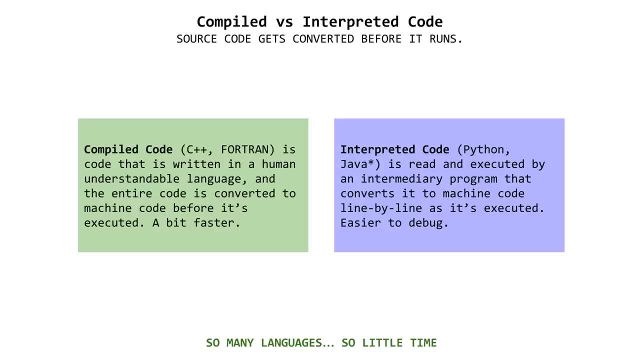 it cuts a few steps out, it's a bit faster, but there's some downsides to that too. it's much harder to troubleshoot because now you can't take it apart in pieces. you got to take about the whole code to find out if there's a bug, and you know people. and it's a lot harder to learn to write. 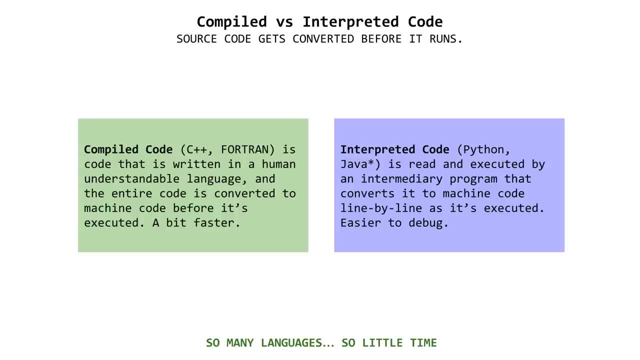 code this way too. and then there's interpreted code like python and java, and uh, there's a java compiler too. but it's just to be simple. it's read and executed by this intermediary program that converts it to machine code line by line. as it's executed, the advantage is it's easier to debug. 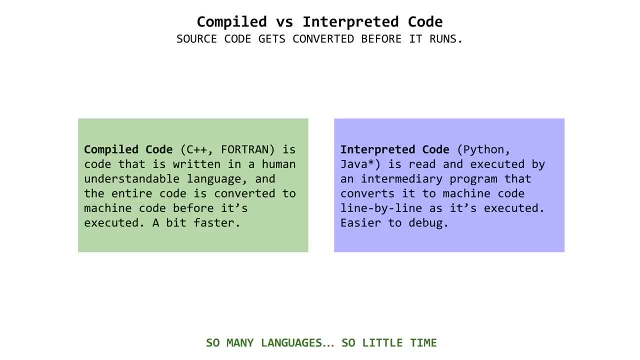 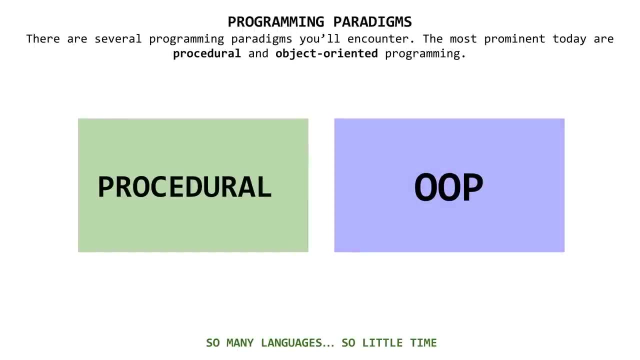 the uh. the con is it takes a little bit longer because there's an extra step in there too. can you notice the difference in speed? usually not. some people say they can, but i don't know who knows. just need to know those two differences, and then there's a couple. there's actually 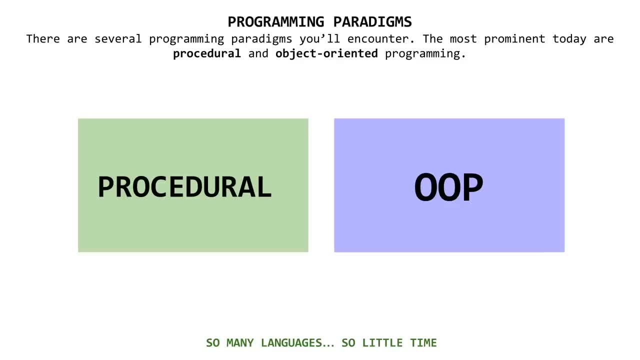 multiples which just narrow them down to procedural and object-oriented program paradigms. so these are the most prominent things you'll run in today. think of procedural like a straight line of code all the way down. it's got to follow these things specifically. and object-oriented programming can kind of spread out the little buckets. you can kind of put things. 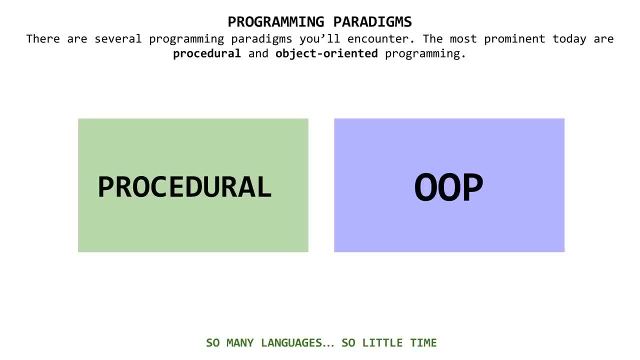 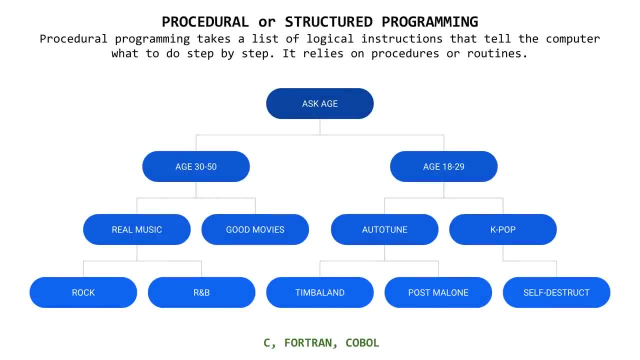 together a little easier and reuse your code. so that's an advantage of that. makes it a little cheaper and a little quicker to write. so procedural. this is a procedural uh example. it's again it's oversimplified, but just a list of logical instructions. the computer follows step by step. so if i follow to the right, i ask rage. if i'm 18 to 29, i like kpop. 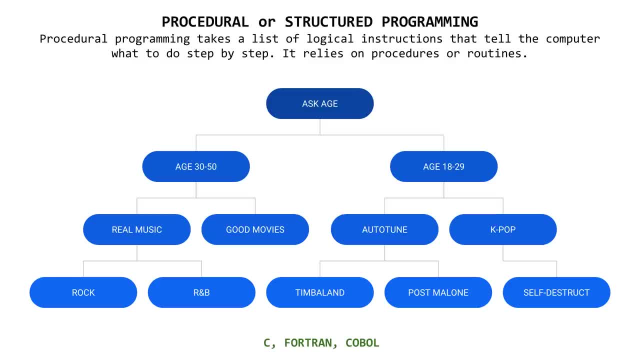 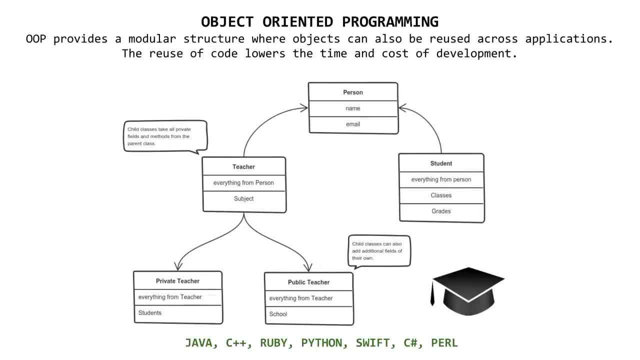 and i'm going to self-destruct the computer, get it machine languages or, uh, procedural languages like c4, train and cobalt kind of go along, that more procedural programming. and then there's object-oriented programming like java, c plus, plus ruby python, all these other ones they kind of take. 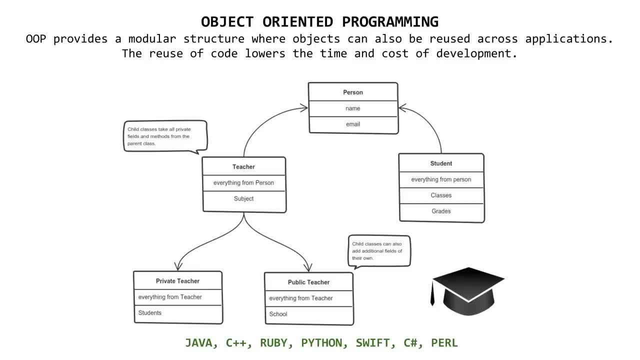 these little chunks where you can use this reusable code to lower the time and cost of development. so most people are learning object-oriented program now because it's a little more- uh, inexpensive and a little easier to learn too. this kind puts everything in little buckets and the buckets 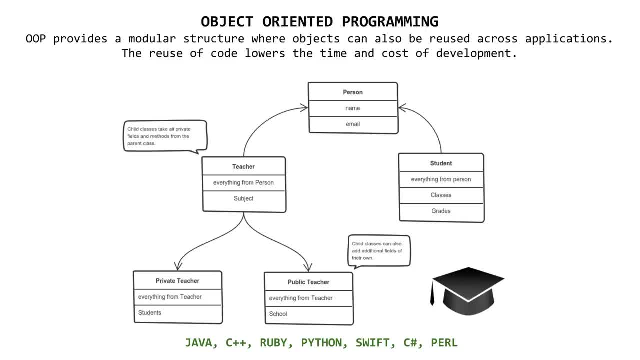 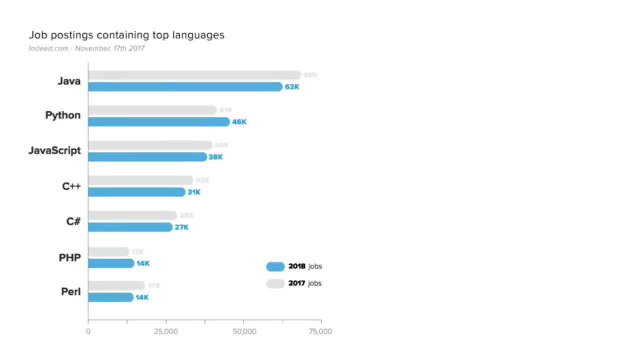 are kind of all assembled together and, uh, handled in neat little chunks, so it makes a little more sense to a lot of people. now, as far as the distribution, according to indeedcom, back in 2017- and this obviously will change- java is the big dog, python, javascript, c plus, plus, but there's a lot of. 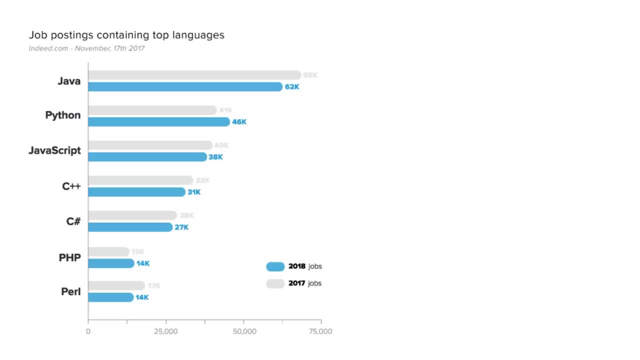 stuff out there, and this is what i'm trying to tell people going to school now that, um, you know there is a ton of jobs out there. it is not the easiest degree to get a lot of people fall out of this thing, because- not because of math, it's just because the logic thinking is. 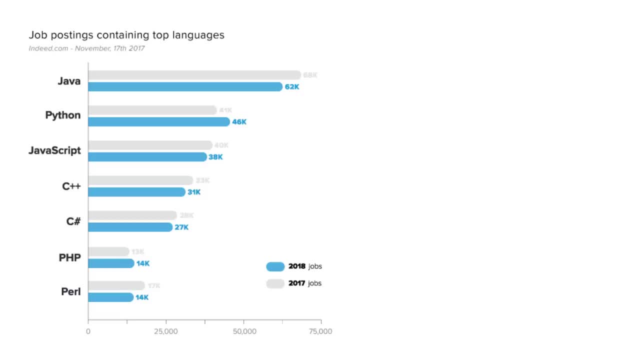 it's kind of difficult. and the other thing about it too is you kind of have to- you don't have to- be introverted, but you know introverts kind of do a little bit better in this profession because you really need to sit down and concentrate on your code, not so much with object. 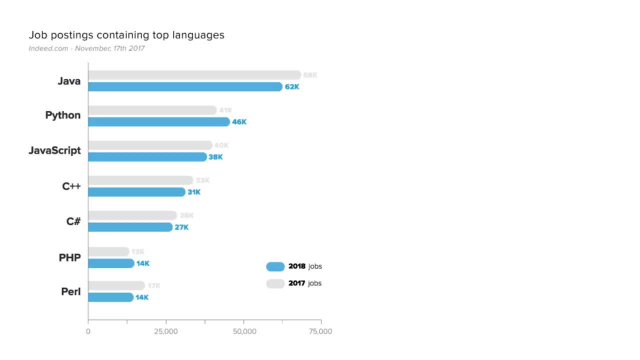 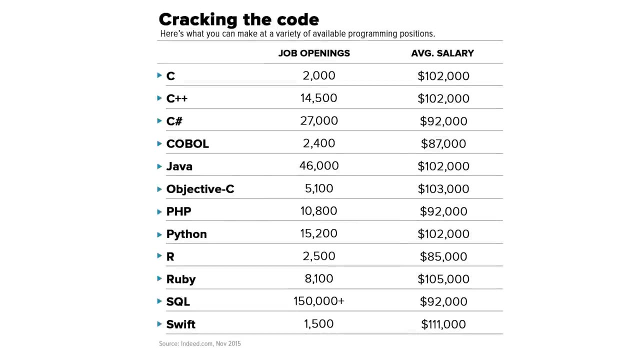 and programming anymore, but the procedural stuff. but uh, yeah, there's just uh. the bottom line is there's a ton of of job openings in uh languages for experienced coders. and look at some of these salaries: man, big money. some of these people make close to this coming right out of college, i know. 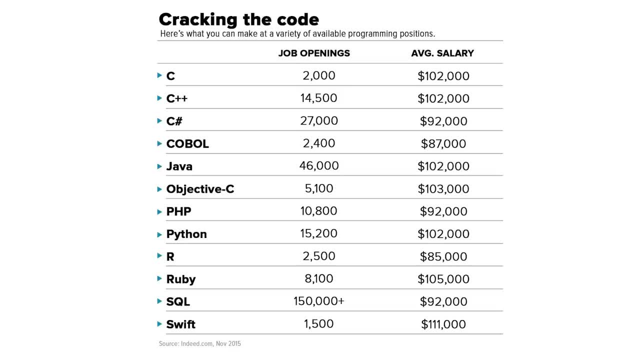 kit came out of college, started about 84 000 a year right out of college- his first job right out of college with a coding degree. didn't really know any of the higher level languages and they taught him everything on the job. but- and this is back in 2015- some of these have gone up too and there's 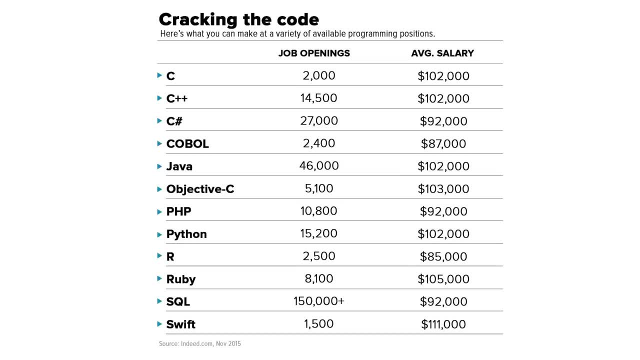 some new languages that aren't even shown on here too big money. it's not uncommon to get a six digit job in uh coding, so it's some good money. it's a great gig and honestly, i don't think it's going anywhere and i think the need for coders is going to increase for the next several years. 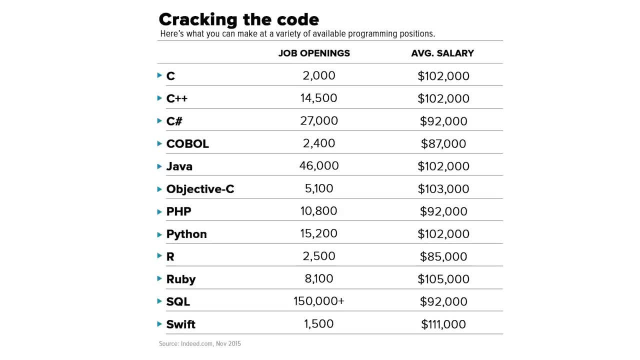 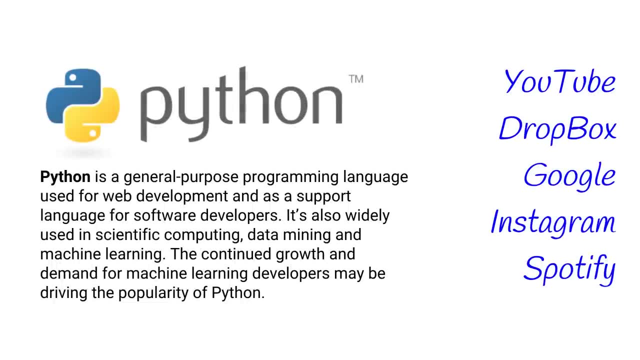 until code learns how to code itself. but i think, uh, we really need to come a long way in ai. i think we've got a decade or two before that happens, but you know i could be wrong. let's look at some of the top level languages, or some of the more popular languages. python: you've seen this on youtube. 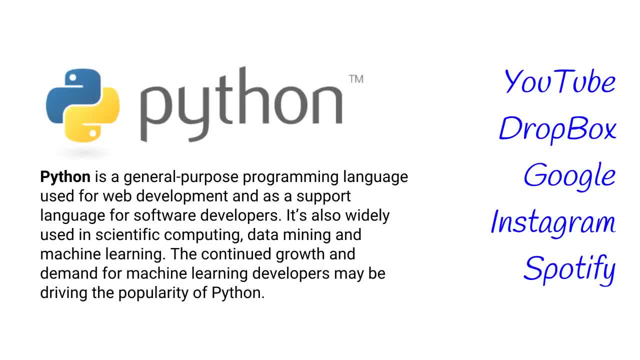 dropbox, google, instagram, spotify. a lot of software developers use this. a lot of people are teaching. a lot of schools are teaching this, now used in scientific computer, data mining, machine learning. it's growing like crazy and uh big in machine learning too. so if you're thinking of machine, 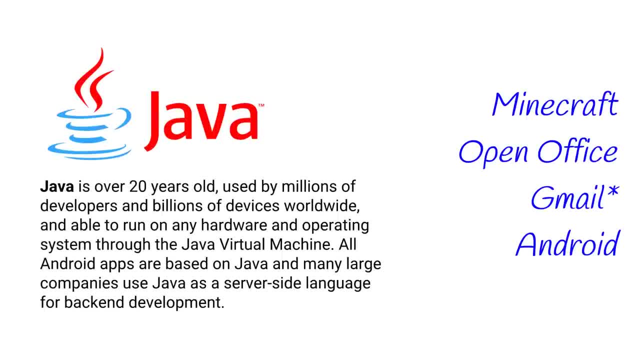 learning, and ai python might be the way to go. nice thing about this is, if you know the basics and enters of one of them, it's not hard to transfer over to another language. basically, their theories and their logic are about the same. some of the commands are pretty similar too, so it's not uncommon to see one person know multiple languages. 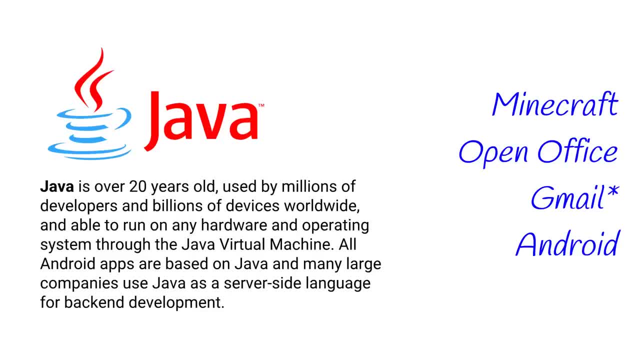 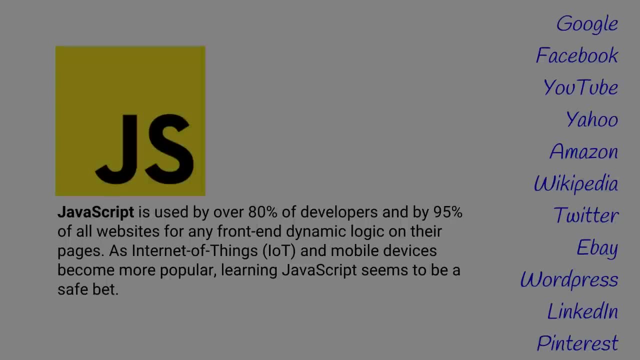 so java? over 20 years old. it's like a granddaddy, used by millions of developers and billions of devices. they call this thing right once run anywhere. all android apps are based on java and many large companies use it. uh, you've seen this in minecraft, open office, gmail uses parts of it, and a lot of android stuff. 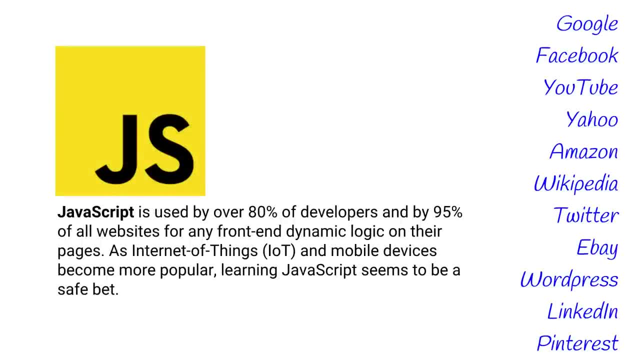 then there's javascript, which has nothing to do with java, just conveniently has the same first name used by a whole bunch of websites today for front-end dynamic logic, for doing like forms and anything that really requires any user input, like emails and stuff, surveys, and you see, this look at. 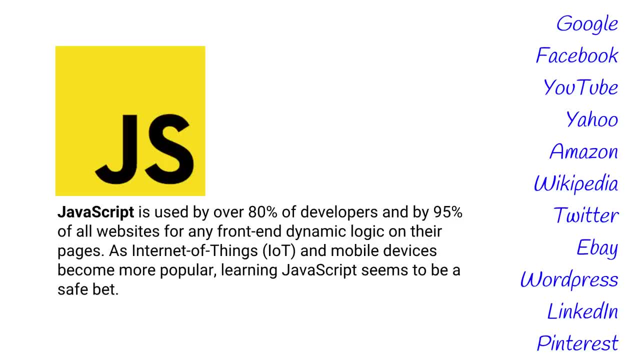 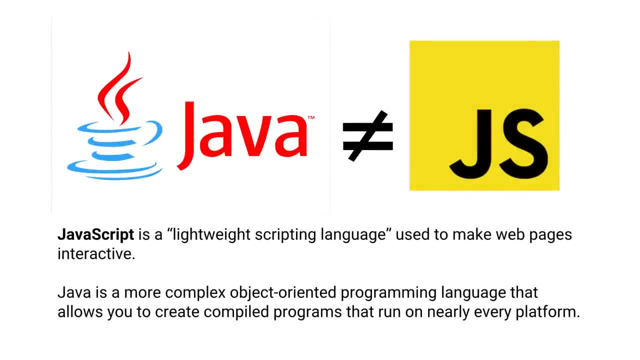 the list on the right: google, facebook, youtube, yahoo, amazon, blah, blah, blah, blah, blah. javascript is every umpire everywhere, great front-end language to learn and a great skill to have in your pocket. again, java is not equal to javascript. javascript is a- they call it a- lightweight scripting language. 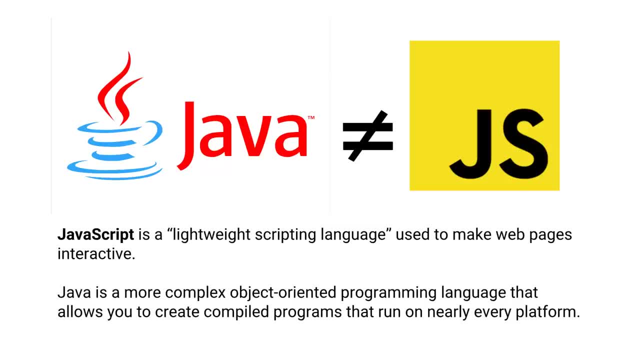 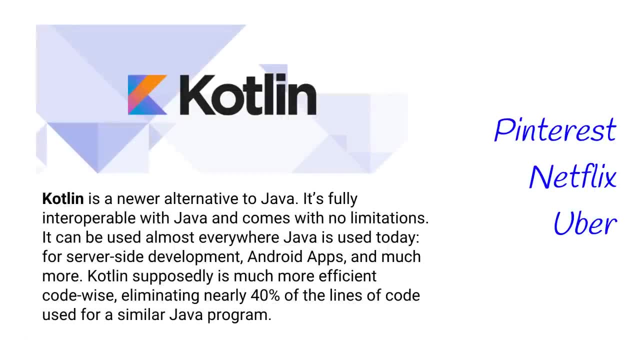 use the make web pages interactive, java's more complex oop program that pretty much could do pretty heavy-duty compiled programs that run everywhere. now an alternative to java is this new one called kotlin, and a lot of people may flip over to this. you see some of it on pinterest. 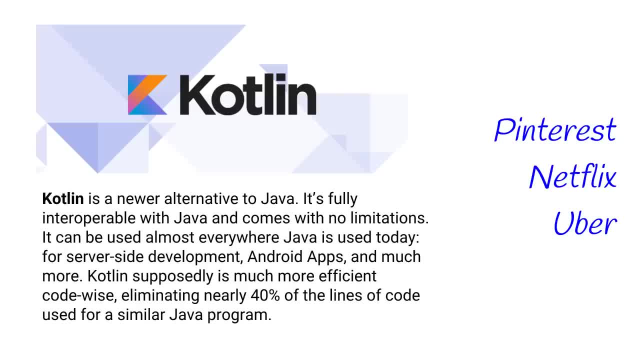 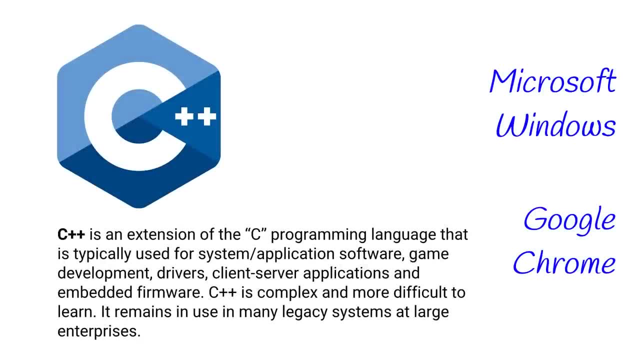 netflix and netflix and uber. it's more efficient. so here's an opportunity for a new coder: learn something called kotlin. see how that shakes out. then there's one of the old, another one of the granddaddies: the c plus plus used actually to code, i think, most of microsoft, windows and google chrome a little. 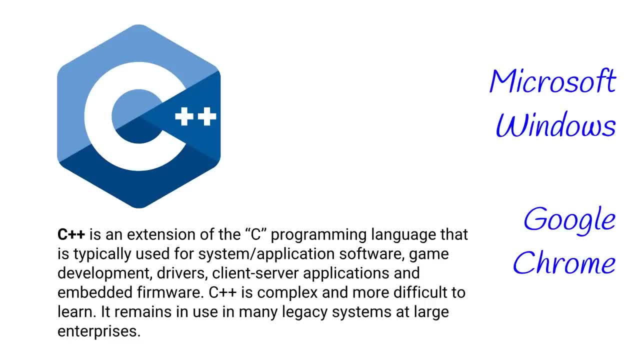 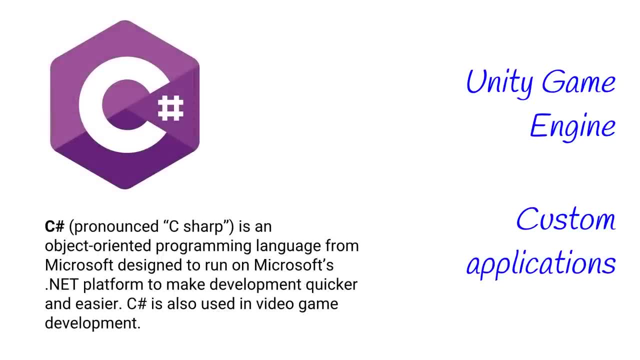 more complex, a little more difficult to use, but uh, it's heavy and it's still in place at a lot of places. you definitely won't be lacking for a job if you've got knowledge in c plus plus or c sharp, for that point. you'll see this in the unity game engine and a lot of people who run. 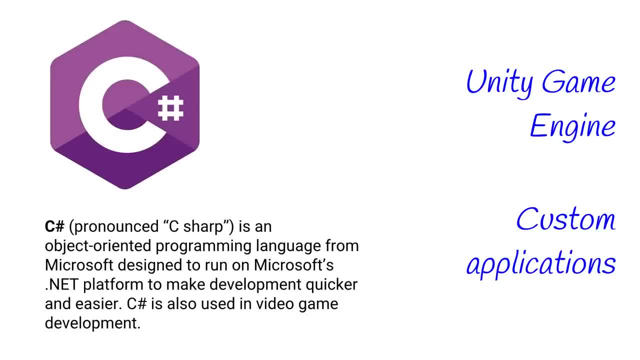 microsoft's dot net platform. that's a lot of big companies. you'll see a lot of internal developers write custom programs like time cards and all kinds of weird stuff, and small companies using c sharp. so another great skill. if you want to work for a big company, then there's pearl kind. 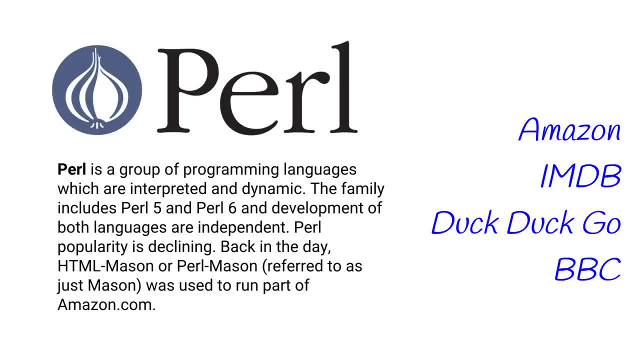 of on the downslide now. it was a big deal 15, 20 years ago. but uh, yeah, it was run part of amazon and imdb. but you know pearl's popularity is kind of declining and people say there's no such thing as a dead language. you know they're always looking for coders to code some of these. 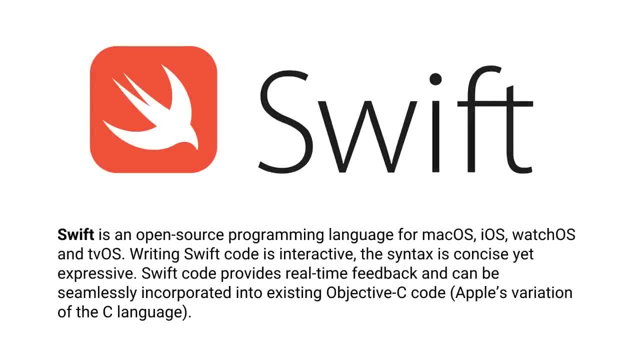 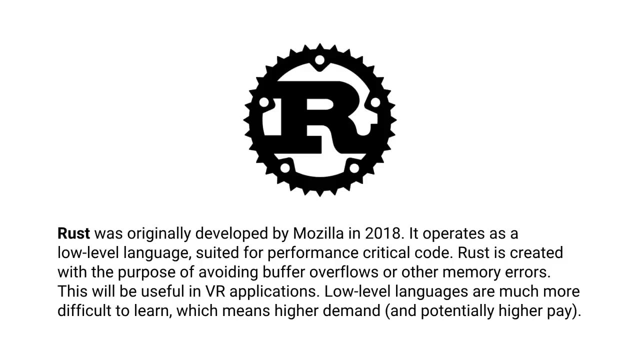 older languages that aren't in favor anymore. noobs on the way up. swift, uh, used for mac ios and os and watch os, so uh, swift code heavy duty. if you're into apple stuff, you want to learn a little bit of swift. and then there's rust developed by mozilla and it's kind of a low level language. 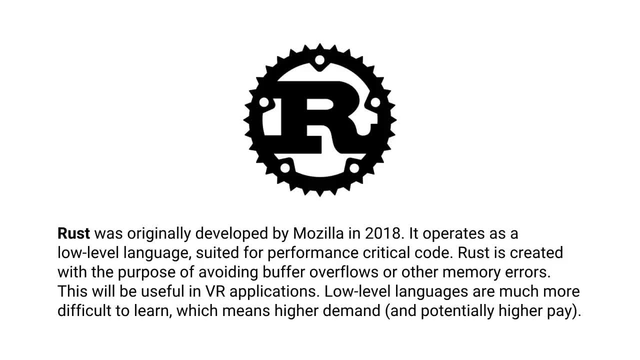 a little more difficult to run but it's highly efficient and, uh, people say it's going to be really good in vr applications that really, really need a lot of processing power, a little difficult to learn but potentially higher pay for rust. and then google come up with this thing called the go, kind of like python, but 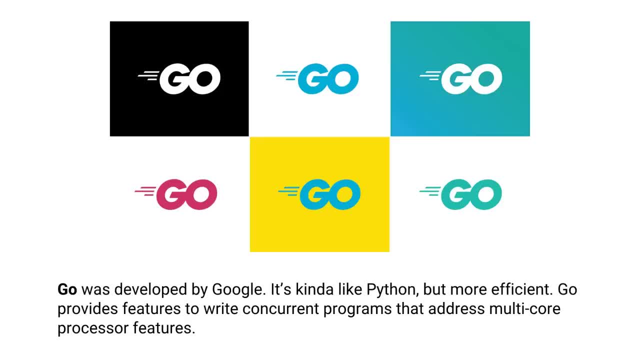 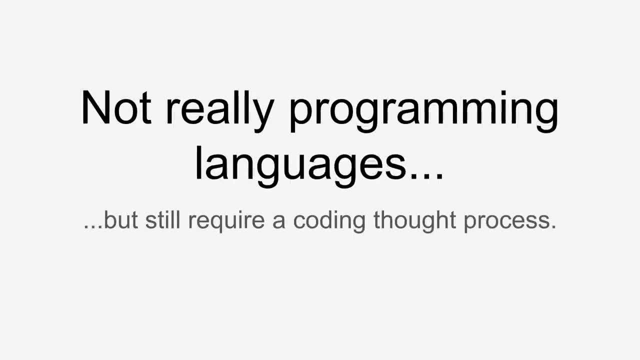 supposedly more efficient and, uh, supposedly this strength is it's able to address multi-core processor features. so you may see this pop up in a lot of games and incredibly analytical programs. so these aren't really programming languages, but you still got to think about it like a code. 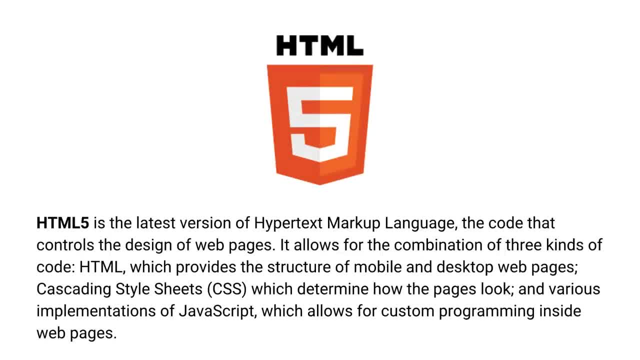 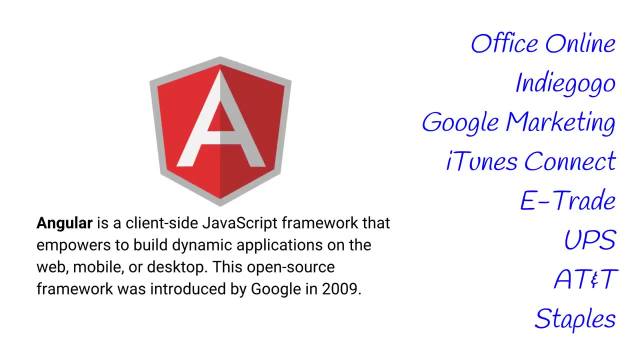 coding process, html5. what most of the web's written on, controls the design of web pages with css and javascript. the html5 kind of ties it all together. so basically everything you see on the web is html5. then there's angular, which is a client-side side javascript framework. it's 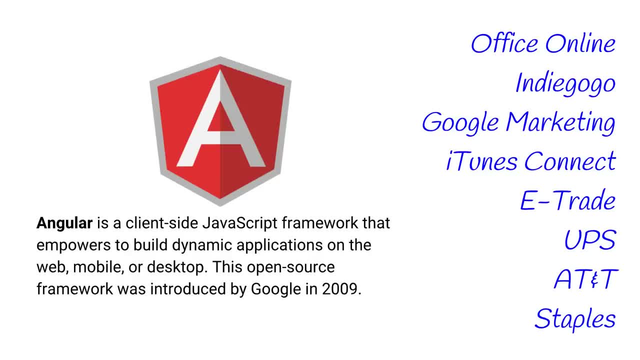 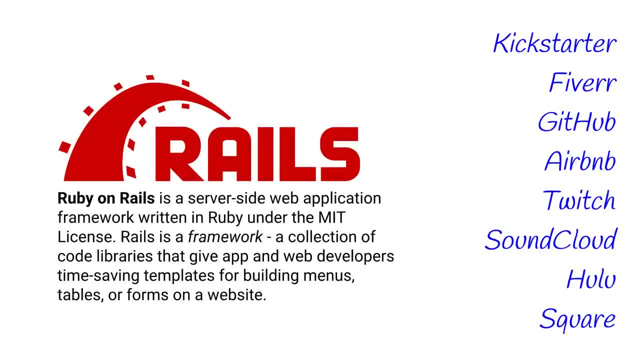 run in places like ups and etrade and at t. it's very, very popular right now and this was actually introduced by google in 2009.. throughput on rails- incredibly popular too. on the other side of that angular thing, a lot of people use this kickstarter, fiverr, github. a lot of people like ruby on rails kind of uh, a little bit more. 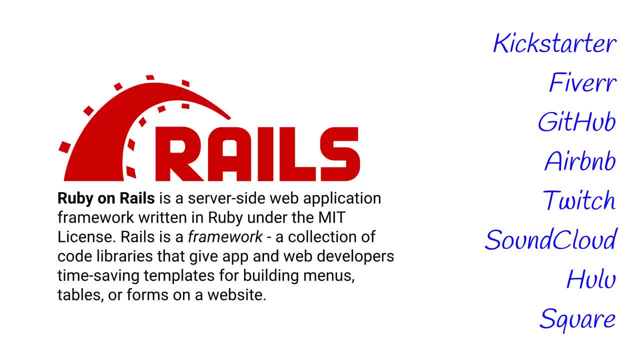 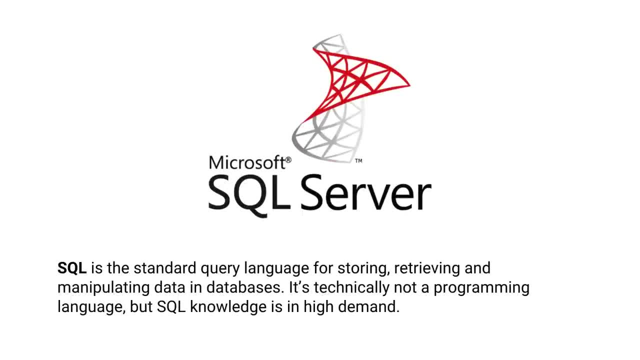 of a framework and, uh, it kind of does the same kind of stuff as, uh, angular, but a lot of people prefer that. and then there's sql. they call it sequel. you don't call it sql because you look like a, like a weirdo, that a newb, so you definitely want to call it sequel. how sql works, to get really good logs on what you need for your software and with descriptions. you got to figure it out, what you're at and how you want to make sure to be able to say: do add javelon to the progress that was in touch with your programs, or how you're working with different software. and 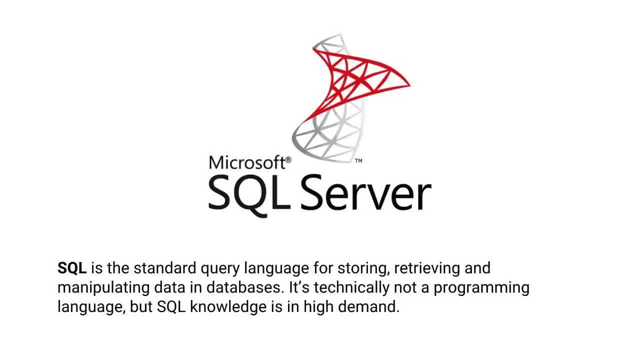 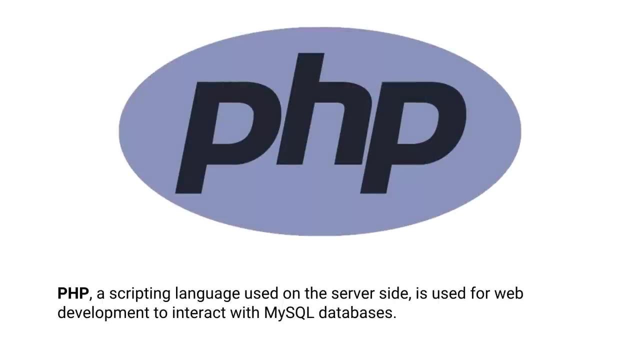 hardware. obviously you'd have to look at things that you can. neighboring and you've got to build in kind of an SQL ends up being SQL. I'll never know, But this is database technology. Anytime you want to store, manipulate information, you're going to use a database. So important to know. Databases will never go away, So SQL is a great skill to have. PHP is used to kind of interact with MySQL databases, So that's kind of important. Still around too. 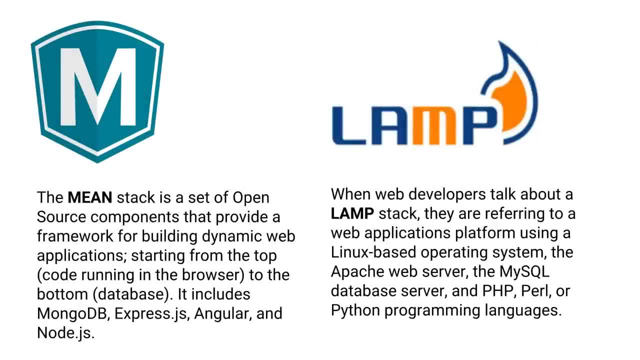 And then there's these new things, Some open source, some not. These are called stacks, And these are used for writing web applications. Basically, programs that exist on the web Don't really need to buy a separate piece of software. You just log into the website and there's your application, And a lot of these are run and managed with something called stack. So mean and lamp are two of the biggies. There's a bunch of other ones out there too, And they're customizable. 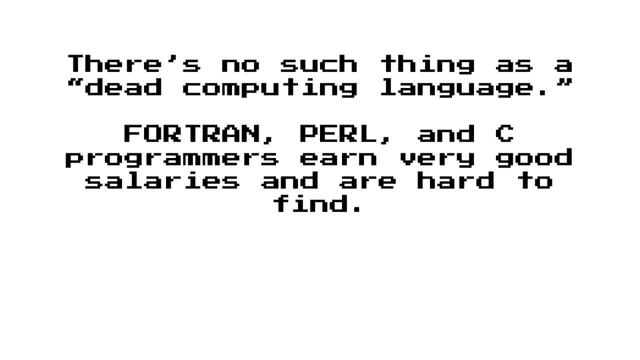 So again, no such thing as a dead computing language. A, Fortran, Perl, C, A lot of those things still running on big companies. I'm putting computers and government computers and it's just unwieldy or too expensive to change. So those coders can end up making some serious money. So don't discount those older languages. 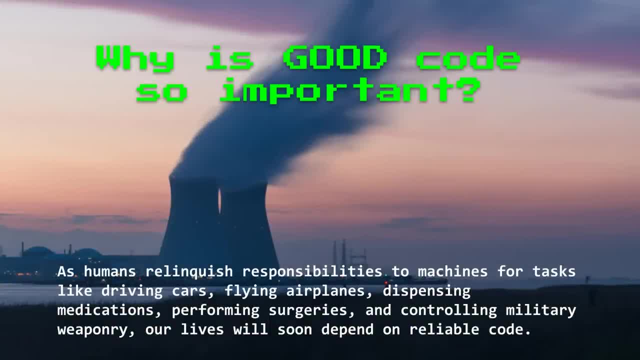 Why is good code so important? Well, as we start letting planes fly themselves, cars drive themselves, Surgeries be done by robots, and even our military running by robots and what they call artificial technology, artificial intelligence or AI, We're going to have a problem. 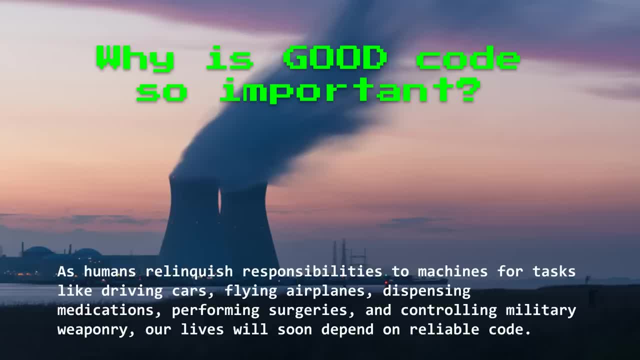 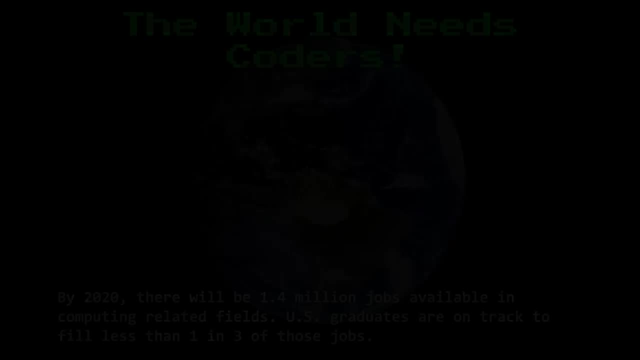 going to need very, very reliable code, because our lives, they already depend on it, but our more and more our lives will depend on it, on the first wave of being directly connected with this stuff. so that's why, more now than ever, code really needs to be tight. it needs to be really really good. 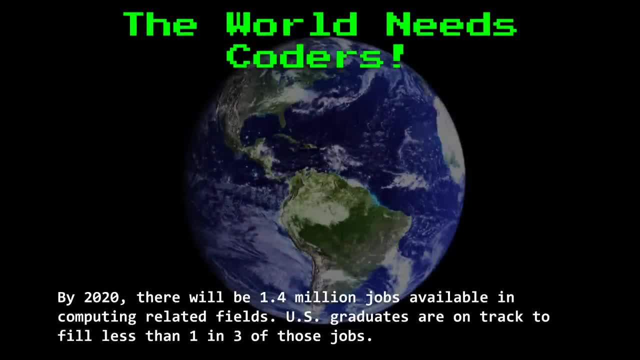 and the world needs coders right now. this is we're in, this fundamental change, this fundamental paradigm shift from human computers, from human thinking, to a world that will soon be thought out, for us meaning ai and machine code and machine. well, not machine code, but machine learning, where machines will get smarter and smarter. we're not talking like terminator stuff. 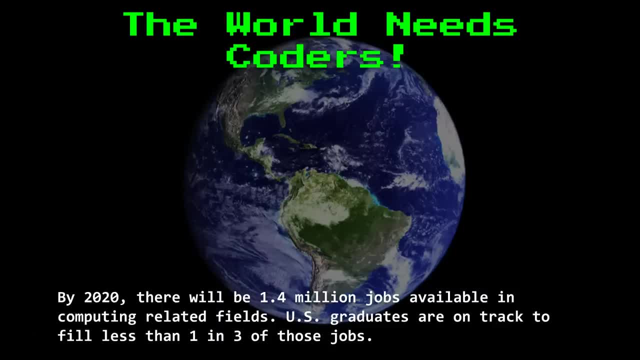 although that is a distinct possibility that people like steve jobs were afraid of, and bill gates has spoke out against. i think elon musk has a thing about it too. but as long as the code is good and you've got safe control guards built into it, we're going to be okay and our lives will be better. These computers will be. 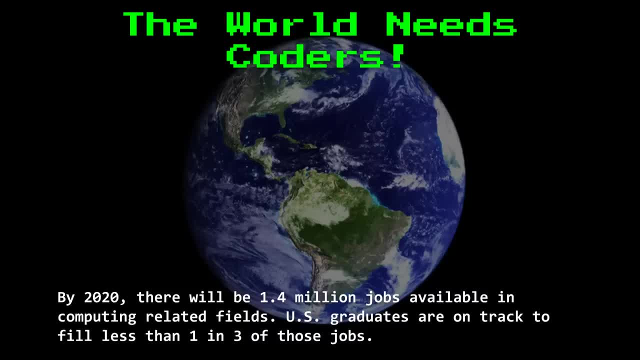 able to think about problems of the world without bias. Well, they'll always have computer the coder, the original coder's bias, but they'll be able to figure out solutions to things that we couldn't think of ourselves. And it's just really an exciting time to be a coder And 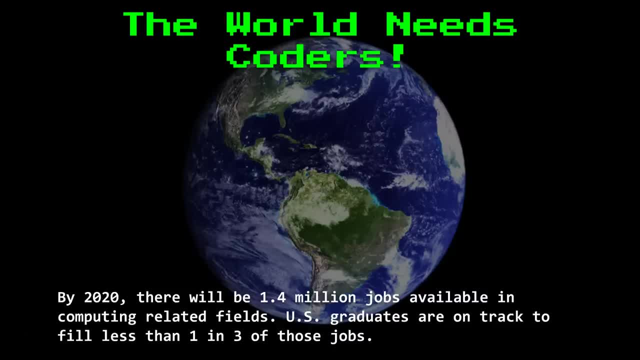 as a student right now. I think it's a great time to be involved in coding and a coding career. Really, really exciting things happening right now. We're kind of at the forefront of that change, of that whole dynamic change. So again, a lot of openings: 1.4 million jobs in computing-related. 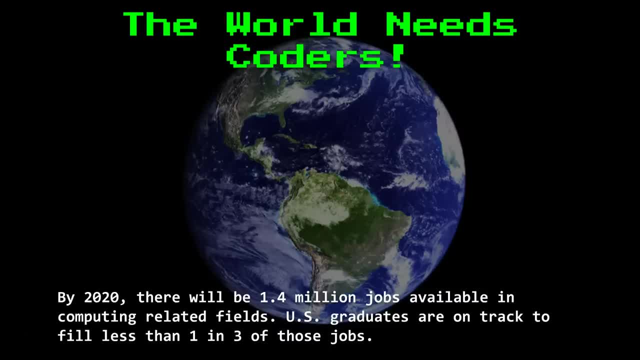 fields by next year And US graduates can only fill one out of three of those jobs. And if you were saying: well, that's great for India and China and even Africa- Kenya's bringing up a whole bunch of coders now, but it's better if those jobs are here so we can supply. 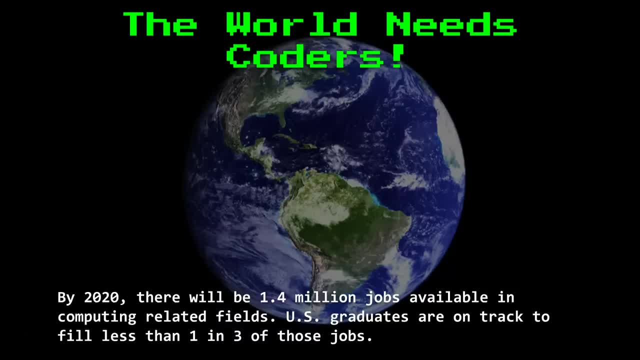 tax revenues, we can build our infrastructure, we can kind of make a better lives right, And I think that's a great time to be a coder For ourselves in this country, in the United States or any country that you're thinking of. 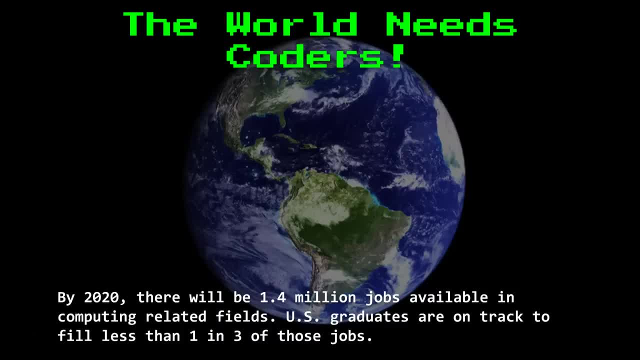 for that in your own country. you definitely want to build up coding education in your own country, wherever that is. But even right here in the US, man, one out of three- we can only fill 30% of those jobs. That's pretty embarrassing. What is everybody else studying, man? 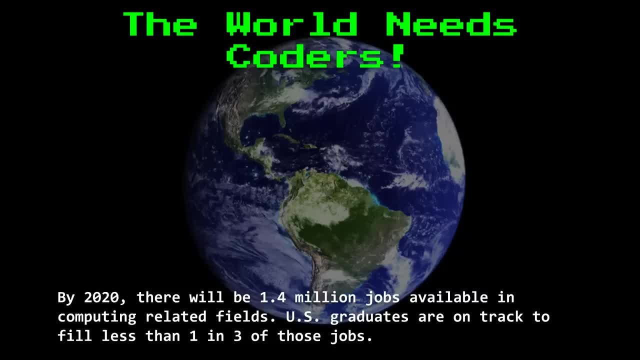 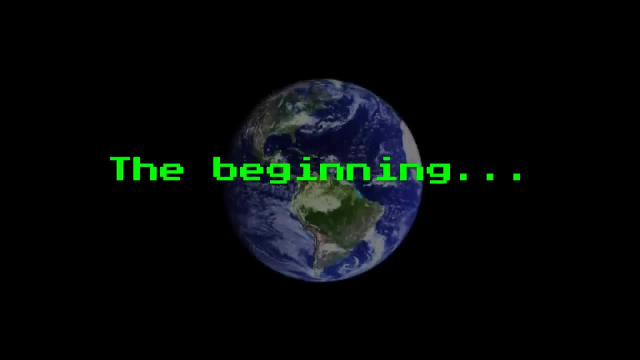 We need to get people on track to learn coding, And that's what I'm trying to do with myself and my kids and my classes right now. So let's get it together. This is just the beginning, people, Let's code, Let's learn to code. Let's make it a better world. 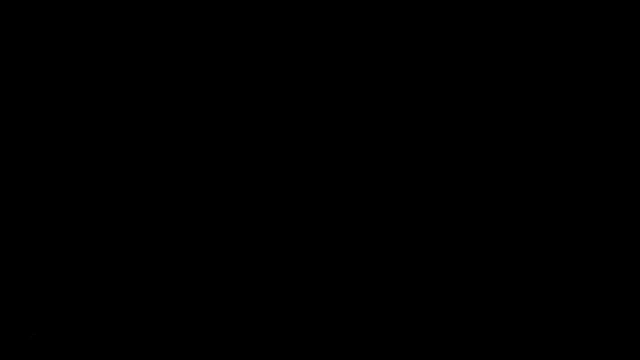 And let's have a little bit of fun and see where this exciting new journey takes us. Chuck Fresh with Computer Care. I'm out. 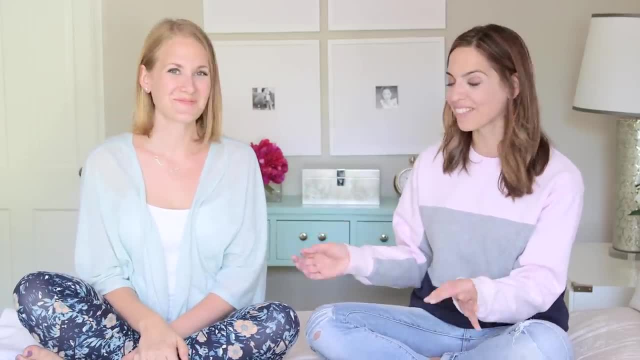 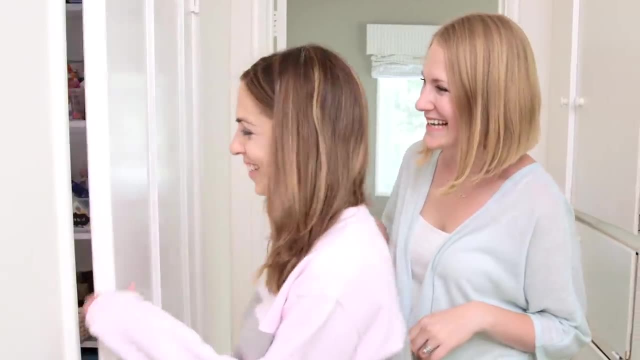 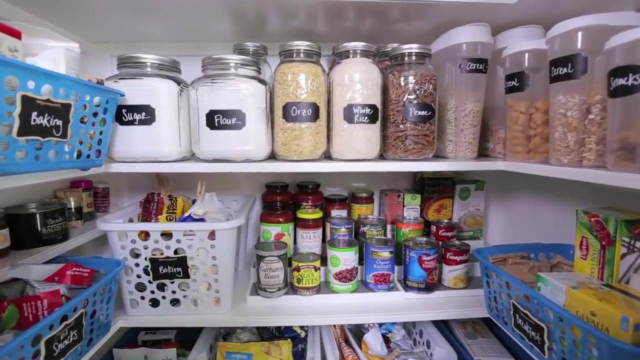 Hey guys. So I was so excited when Katherine told me she was coming to visit and then immediately I was like: oh no, please do not look in my closets or anything we organized together. I'm hiding behind the door. Not how we left it. I call it Yorganized YouTube organized. 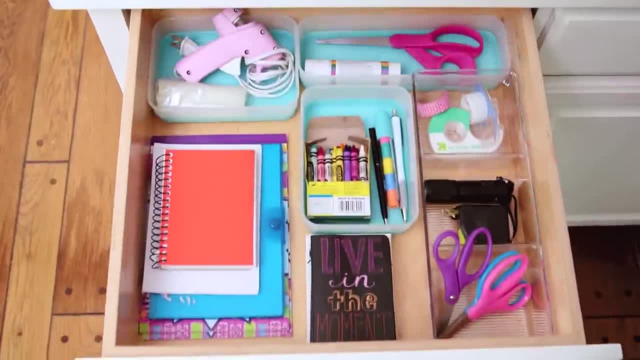 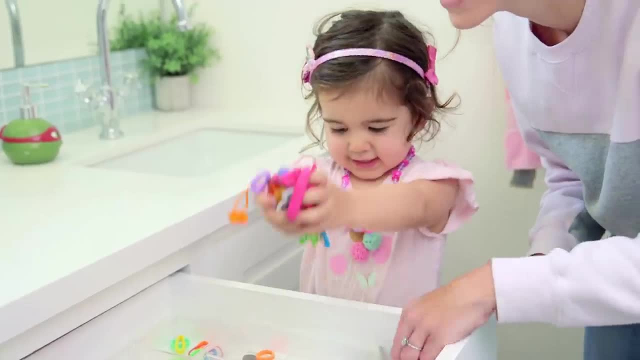 Oh, that's awesome. It looks perfect on camera when you first do it, but it totally needs maintenance. Yes, and I'm glad you guys get to see that. So today Katherine's gonna help us with five tips on staying organized. after you have organized, Just do not pan down Whatever. Nope, Hey. 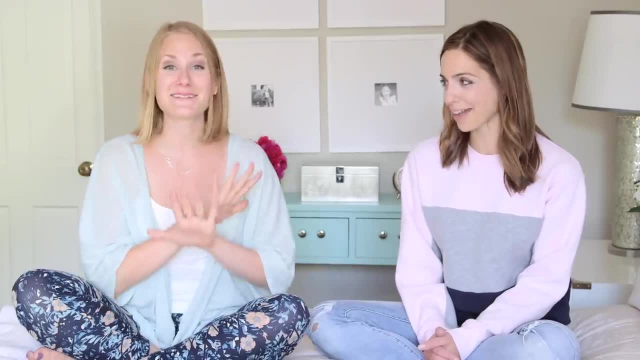 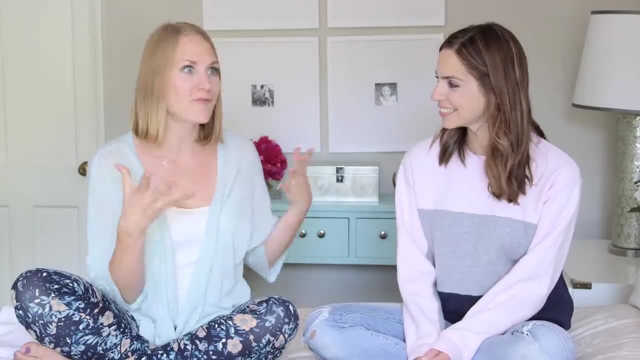 So the first tip is to expect maintenance. It is not your fault, the system has not failed. you Look at Ford snack Some nice sandpaper. If you touch a spot five times a day, like your pantry, expect at the end of every month to have to go in and address things and less frequently access. 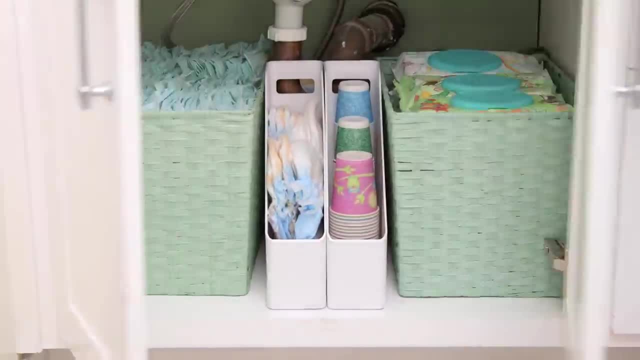 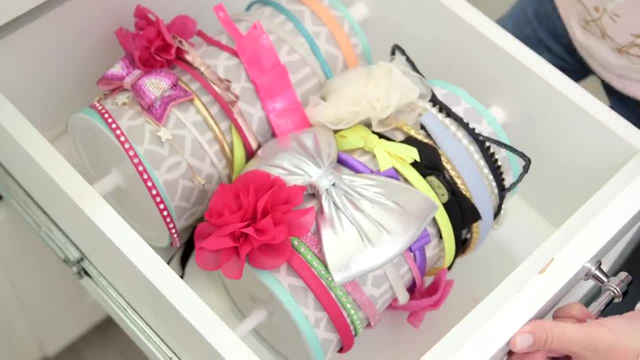 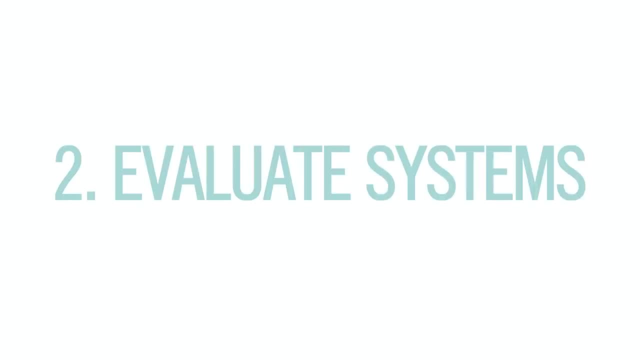 Speaking of the kids bathroom has held up so well. I didn't do anything that looks like this, except for the top door, because we use it so much. Number two: evaluate systems. I noticed in your hall closet that there were lots of lids off of. 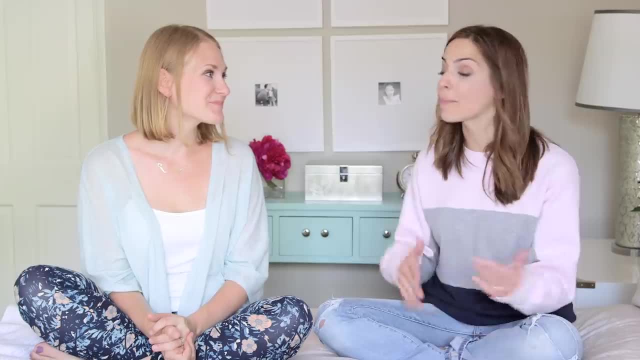 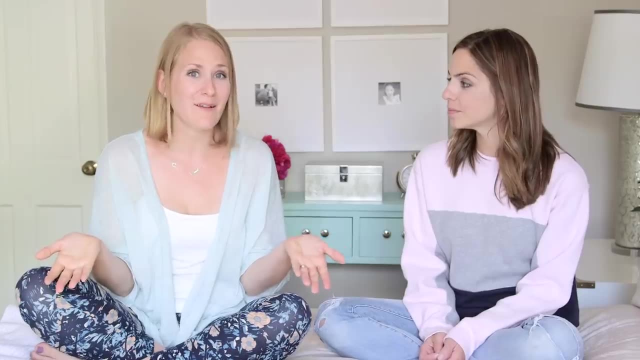 the first aid stuff, Oh yeah. Well, you know my kids, when they're hurt I'm like rushing in there grabbing things. I don't have time to put it back on. So ditch the system, Take the lids away and just don't plan to put anything else above it. so it's gonna actually work for you. Yeah, and then in.